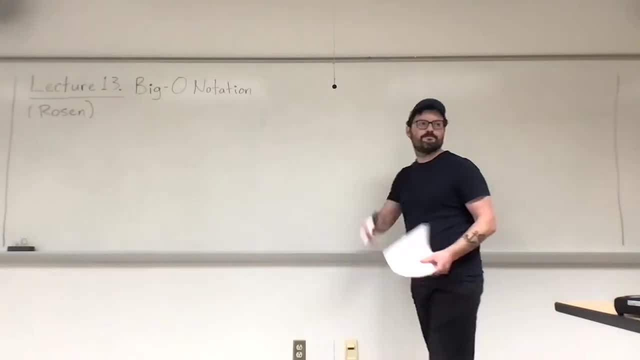 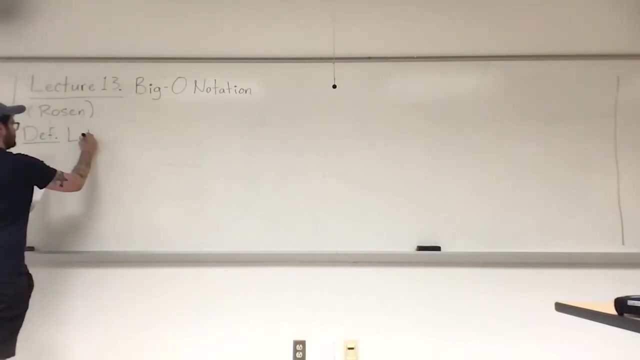 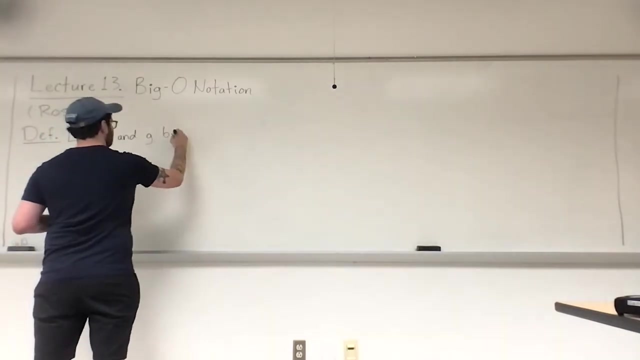 It's different conventions for things. I prefer Rosen. Okay, so there's a definition that's going to kind of guide the entire section. It's a definition. It's going to take me a second to write, So let f And g 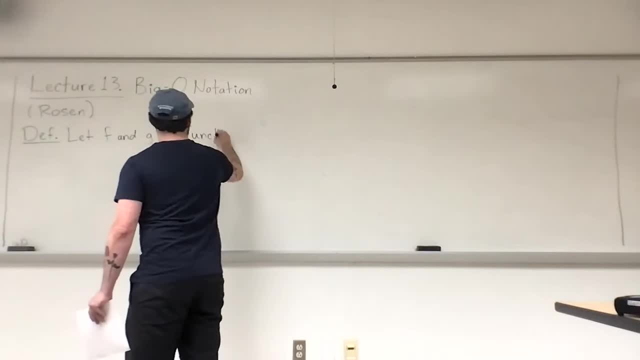 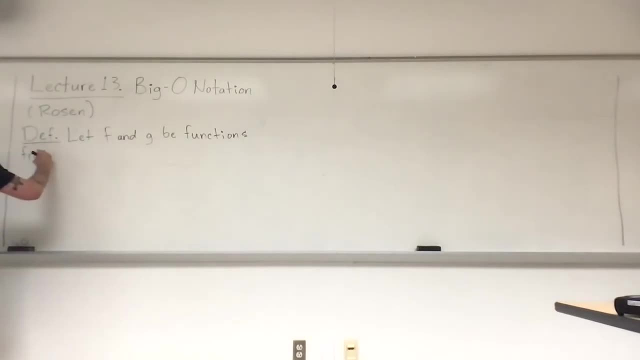 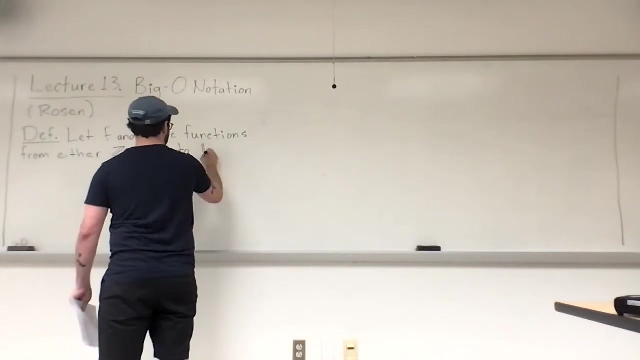 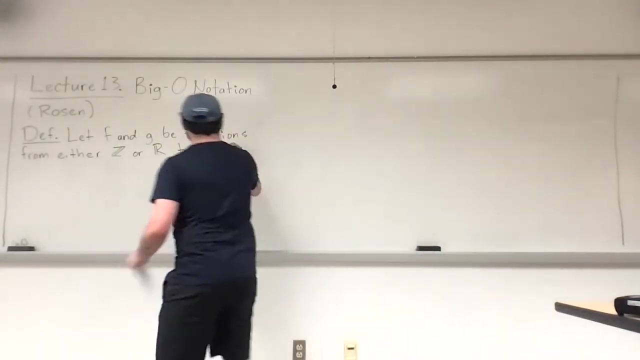 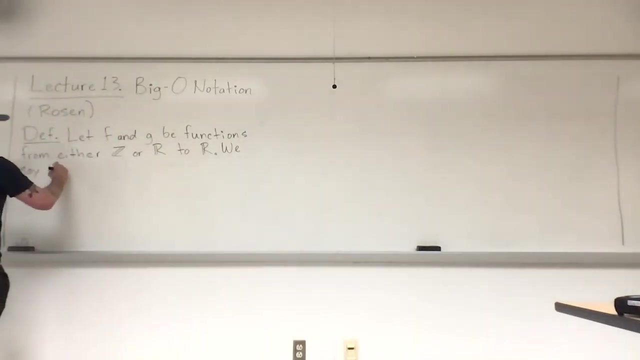 The functions From Either The set of integers Or the set of reals To the set of reals Or some like subset of reals. So We say That f of x Is Big O. 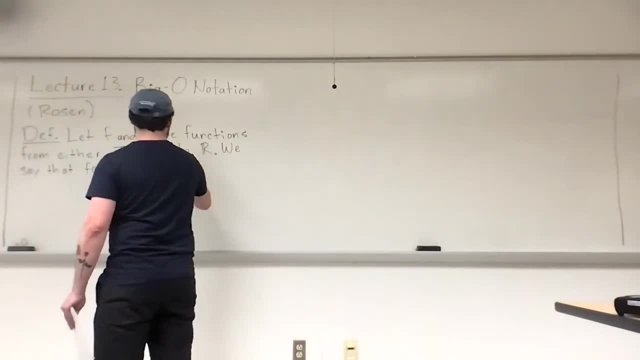 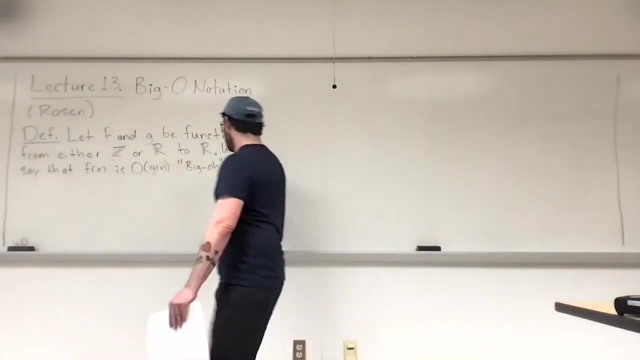 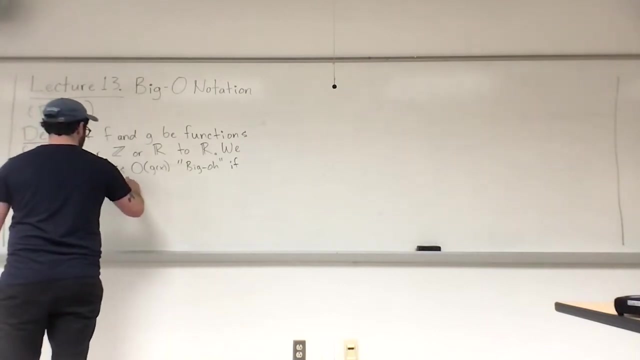 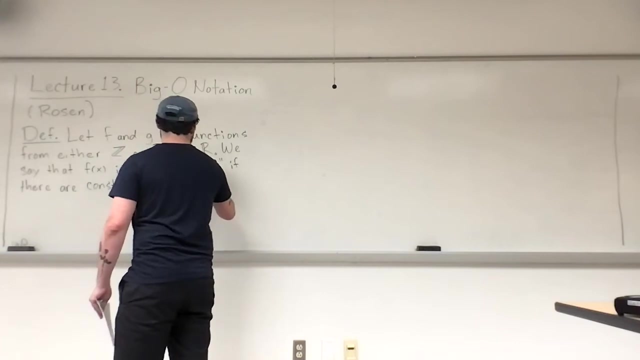 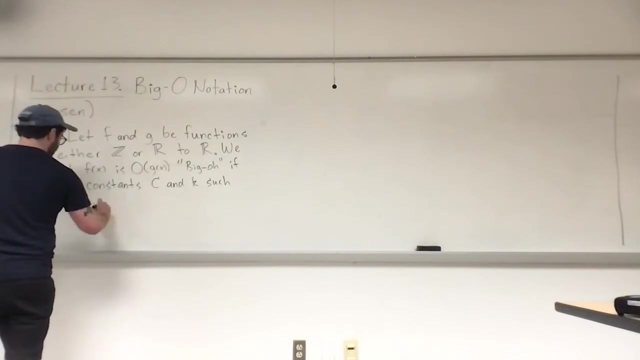 g of x. So this is Big O, So big O g of x If There are Constants, Capital C And lowercase k, Such that In magnitude, So the absolute value of f of x Is at most: 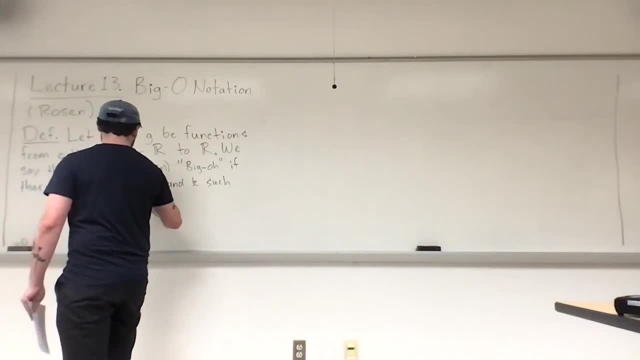 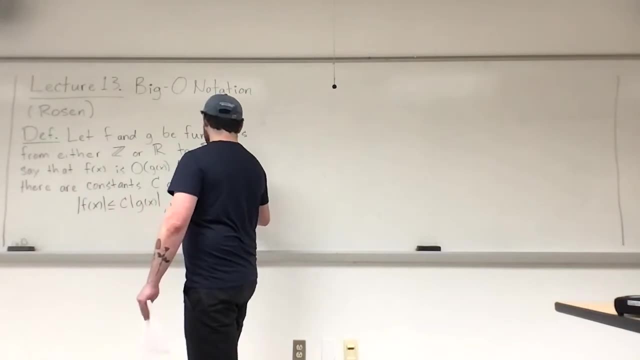 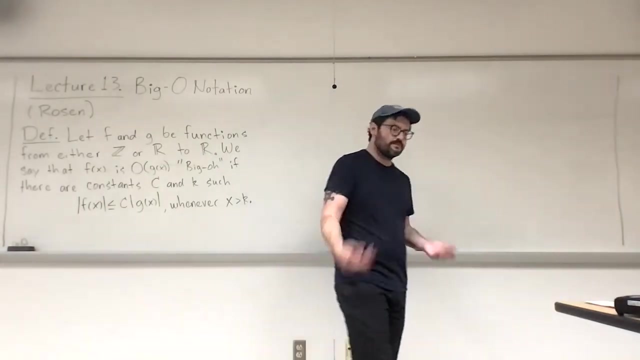 C Times the absolute value of g of x, Whenever X Is greater than k. Okay, So this is a Inequality, And I- It's my experience, Um With Math majors, CS Majors. 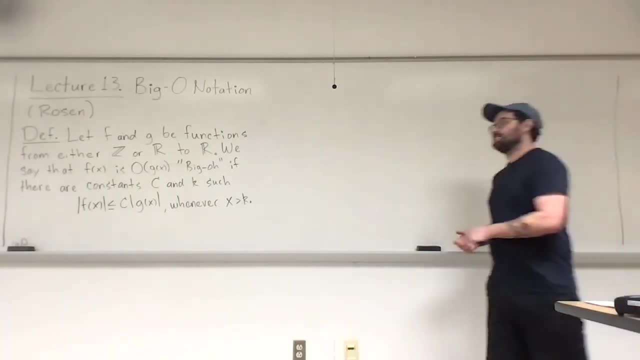 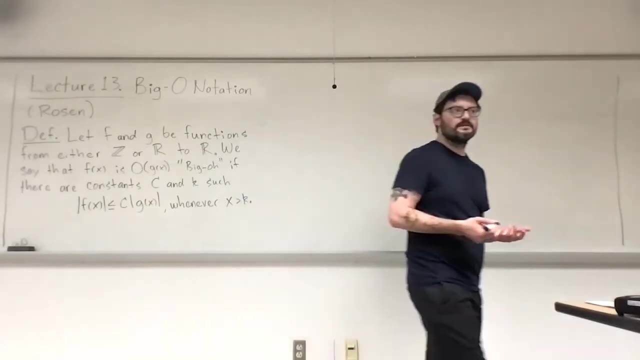 Regardless of like What year they are, That Inequalities are. They seem unnatural To you. Like you're, You're so used to working with equations in Your math courses That inequalities might seem a little bit off. 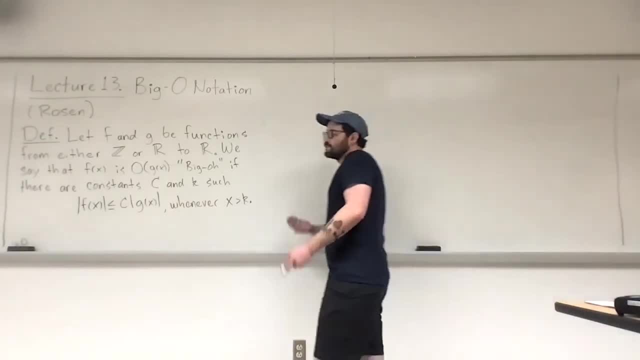 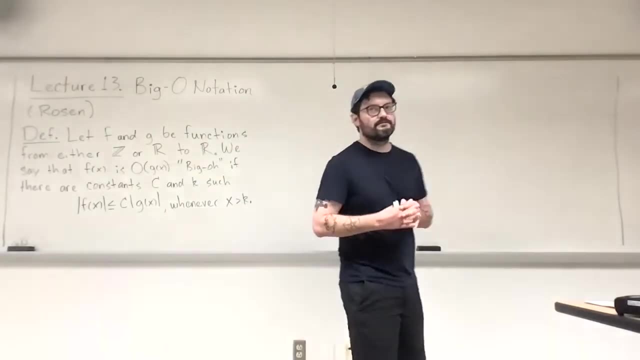 But realistically, inequalities are More common in real-world scenarios. Like most, things are too complex To get an actual equation, Or At least like With With Relation to data. Um, So the best that we can do, 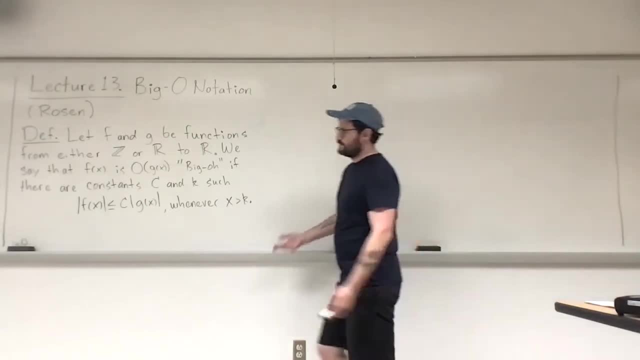 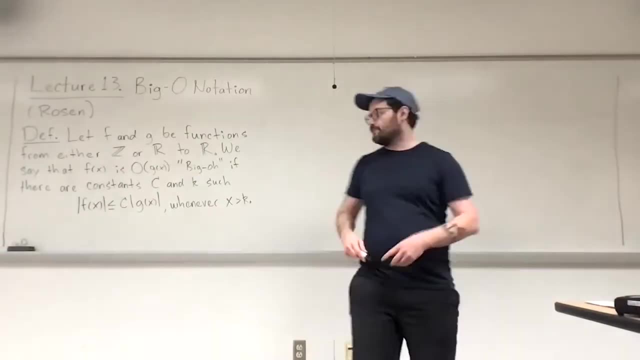 Is bound Things. So This is a bound, Right? So That less than or equal to that Is a bound on This thing's value, Right? So What this is saying is that, So if f of x is: 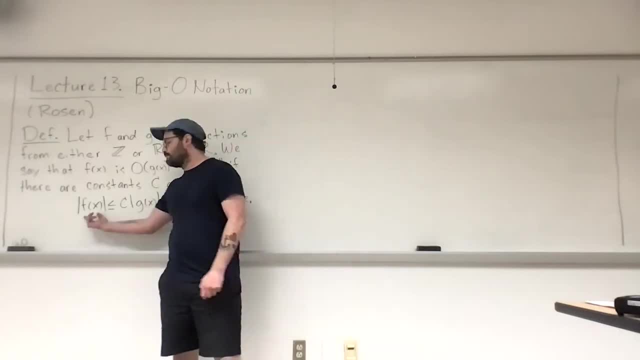 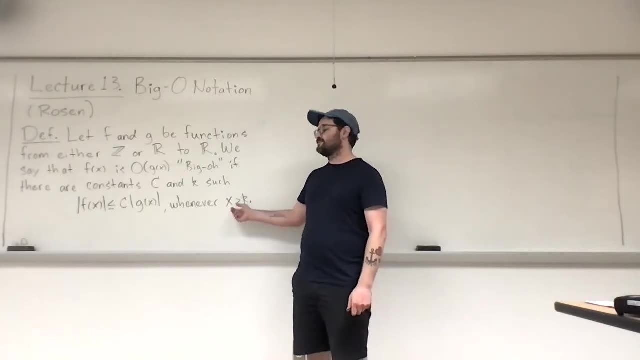 Big O of g of x. Then, Like in magnitude, Is x is increasing Right At some point. So there's like a cutoff k Right At some point For all x greater than that cutoff, The magnitude of f is no more than a constant times the magnitude of g. 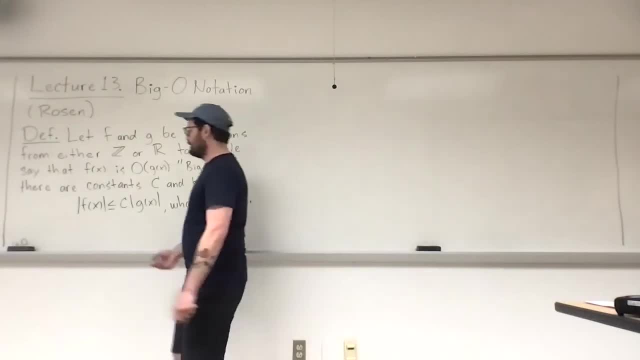 If there's some cutoff where They're no different than a constant multiple, Okay, Which, If they're no different than some, like constant multiple of each other, Right? Like this one's? No more than x, Right. 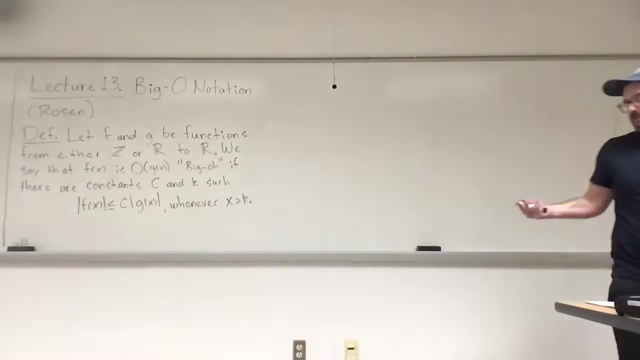 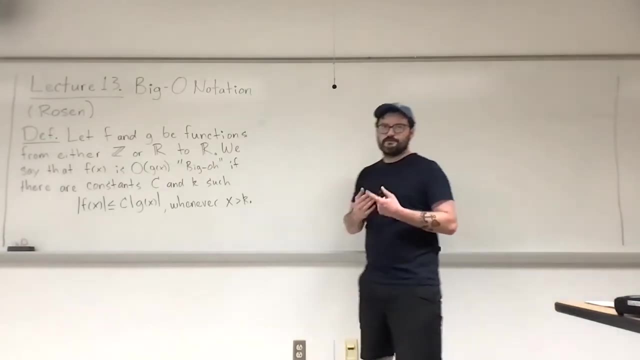 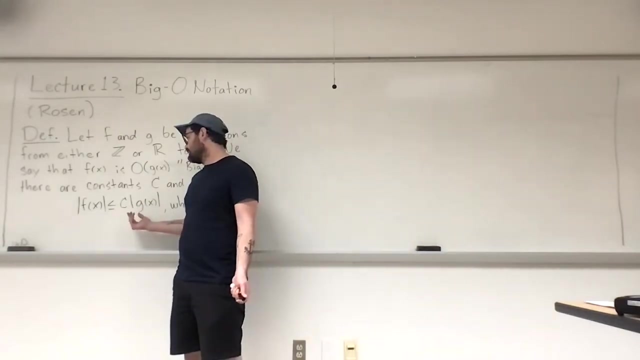 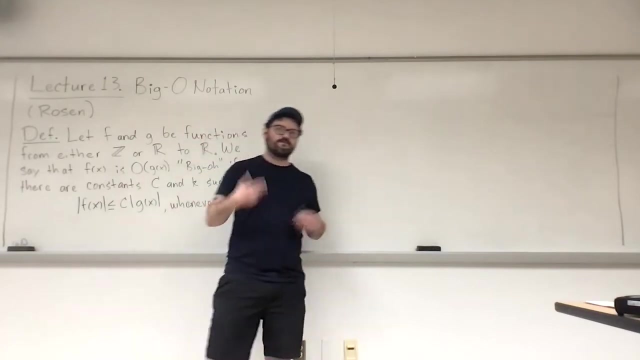 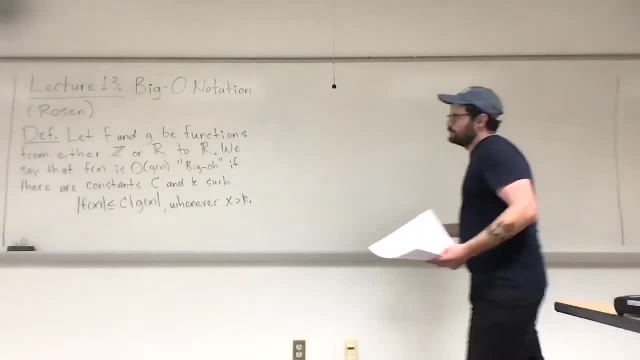 If, Then Then We have a way of like saying: like This one. We have a way of describing this one's behavior in terms of this one. That's the whole point of the idea. So Let's look at an example. 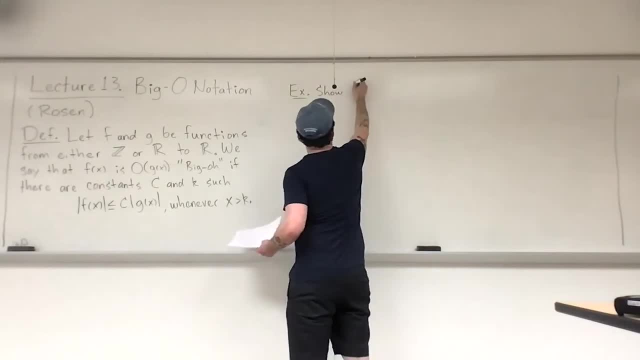 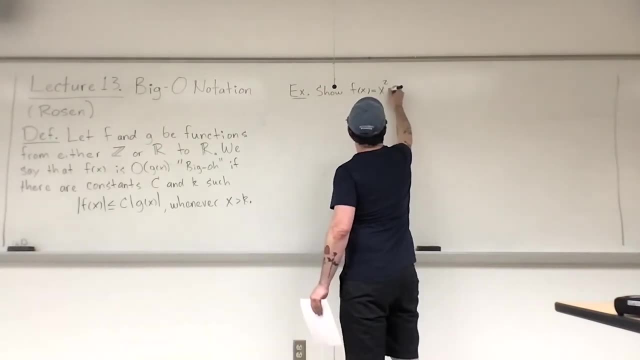 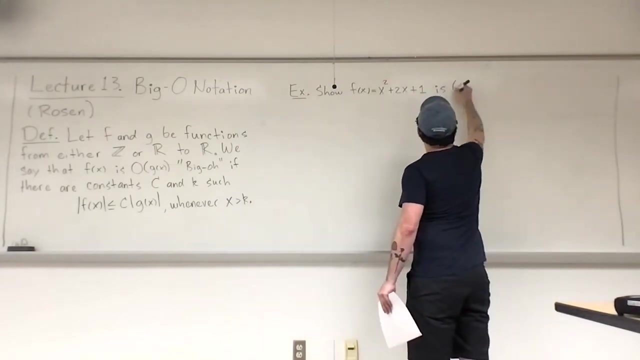 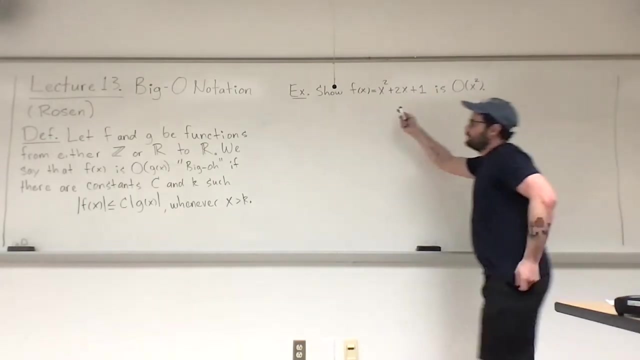 And we'll do several examples. So show: Um F of x Equals to My function. Next, x squared plus 2x plus 1 is big O of x squared. Now, before I work through, actually showing that that satisfies the definition here. 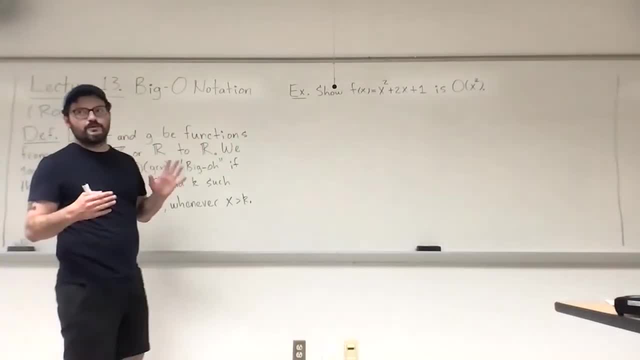 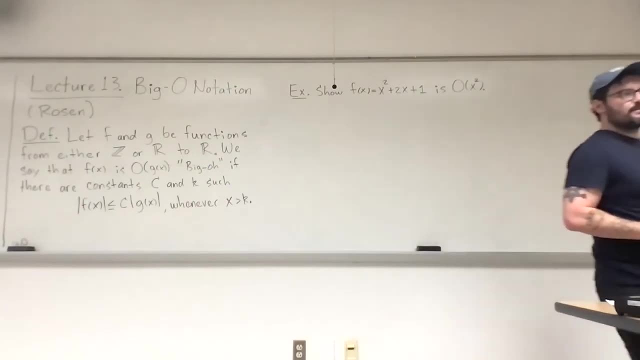 I like to encourage my students to kind of look at it and think for a moment about what happens as x gets really big. So imagine x is like huge. Like let's just say not even that big at first. Like let's just say, like x is like a million. 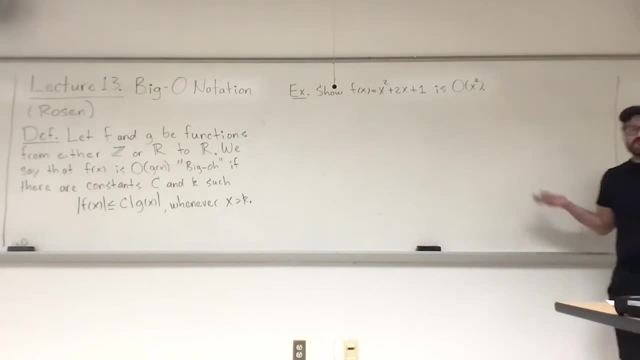 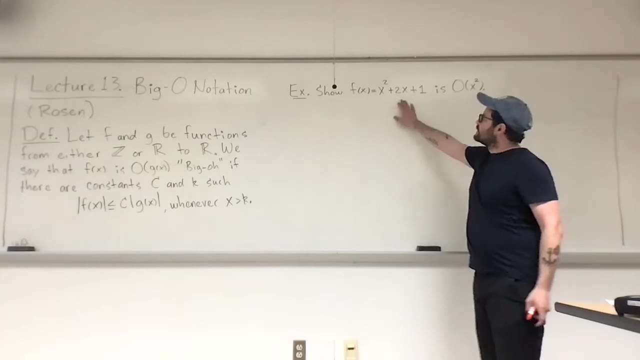 It's not that big of a number, right, It's just a million. There's much bigger numbers, But let's imagine that x is a million. right, This thing here, right, Like, does that 1 really matter when x is a million? 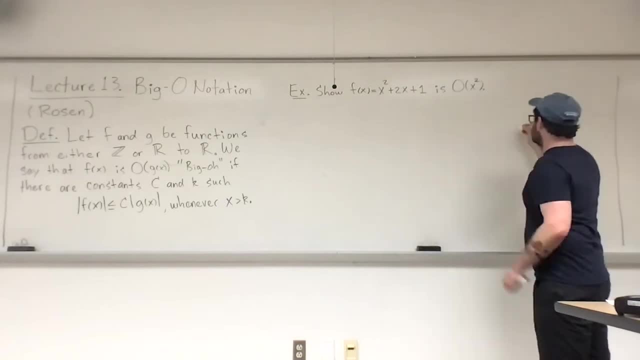 No right, So like I'm going to erase this in a moment, But like x squared plus 2x plus 1 is like approximately x squared plus 2x, right When x is really big. 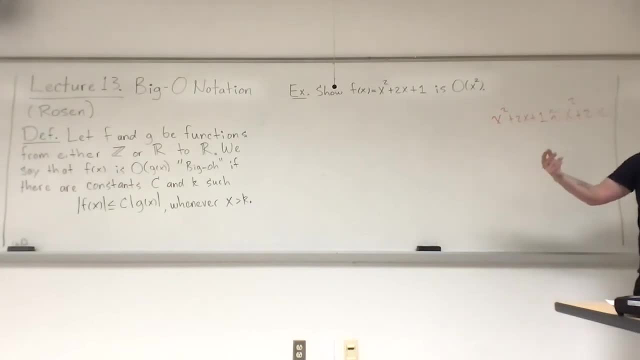 But even then, like, if x is like 2 to the power of a million, that's like way more atoms than there are in the universe, right, Huge number. That number squared Is going to be so much larger than 2 times that number, right? 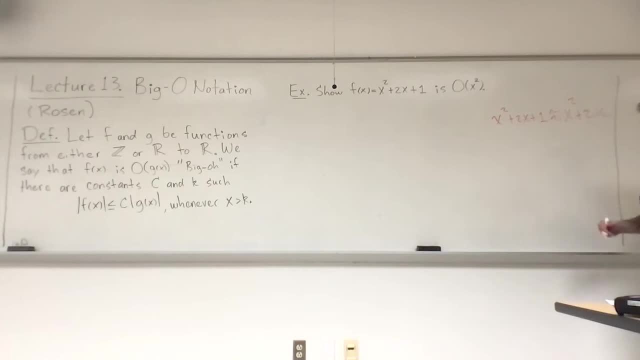 It's essentially the same thing. So then if x is like really really big, then it more or less behaves like that function. It can behave any kind of way when x is small, But as x goes really large. that's where we want to know like: 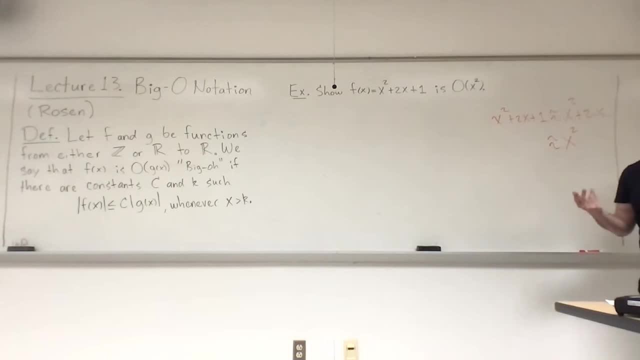 it's almost like considering what we call like the asymptotic Behavior of the function as the inputs get large. What is it behaving like? okay, So even before like proving that that is bigger of x squared, I already have an idea that when x is large, these kind of behave roughly the same. 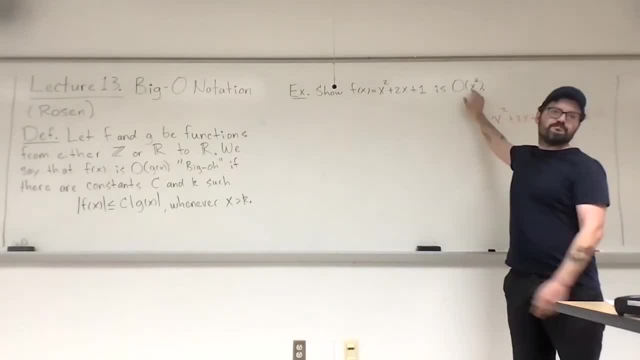 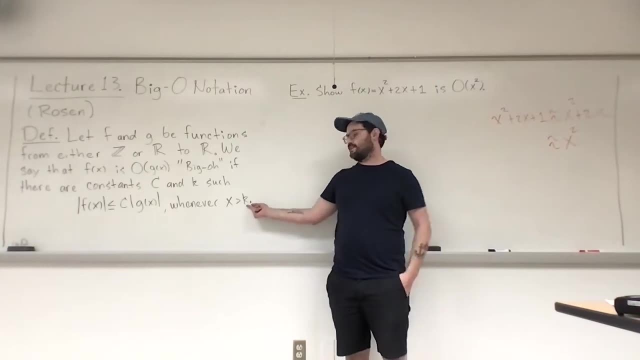 So it would make sense that maybe I could bound that one from above by some constant multiple bet At some cutoff point, right, And the cutoff point is that k, Like for all x greater than that k it's going to, they're going to be bounded in this way. 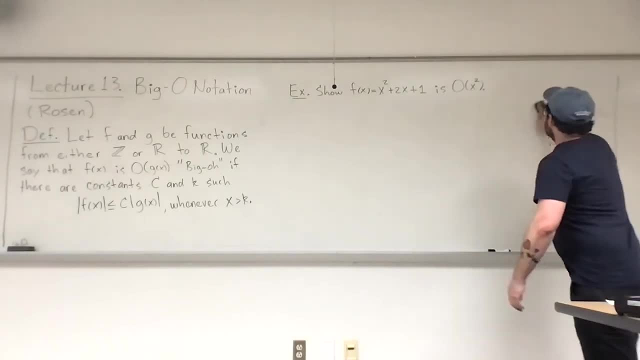 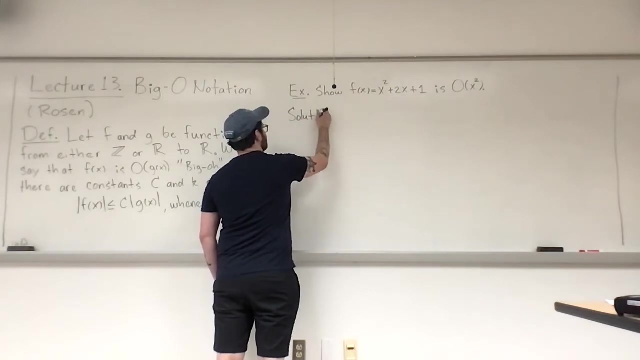 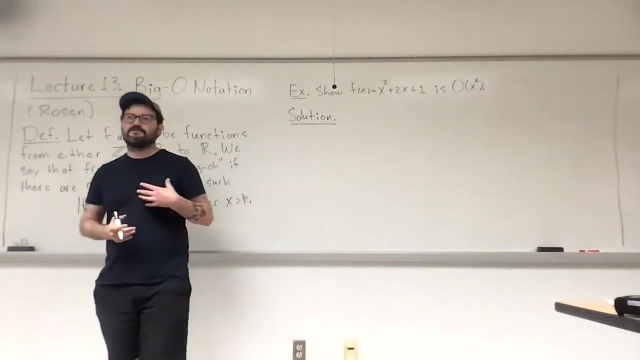 Okay, Hopefully, Okay, So before. well, no, I don't have to write it yet. We can do this one without what I was thinking. So let's look at the solution for this. So before we wrote the solution, we kind of gave ourself an intuition as to the behavior of that in relation to the other one. 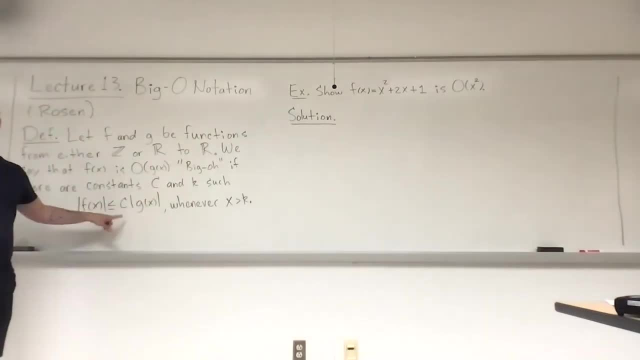 So now we're going to try to show that there are indeed constants like this: Okay, And if we can show the existence right, The existence of c and k, such that this holds, we're good. So let's just look at like: okay. 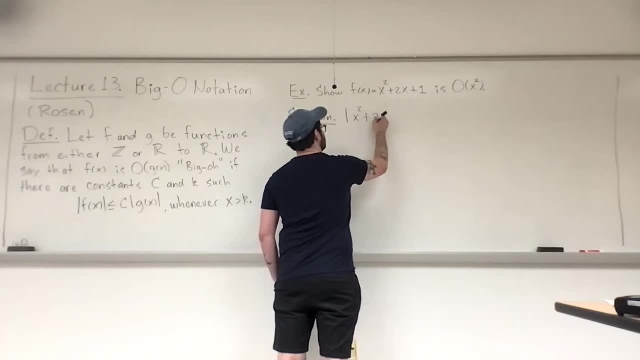 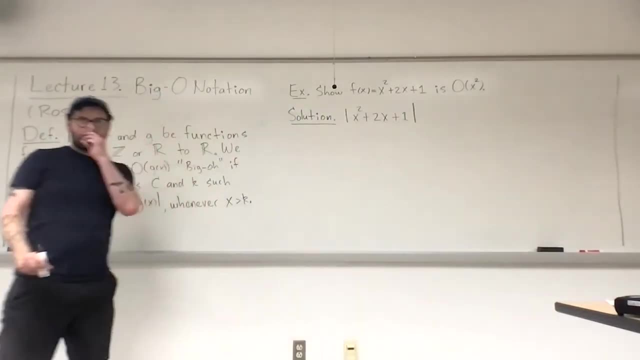 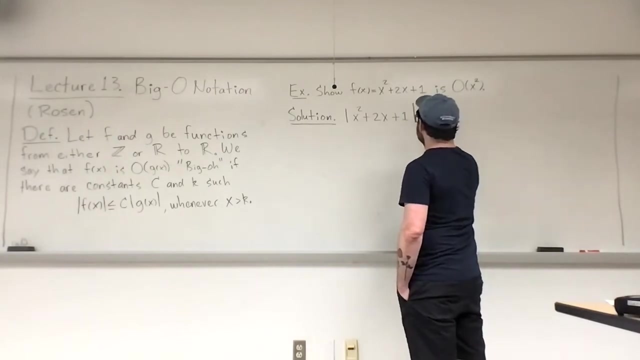 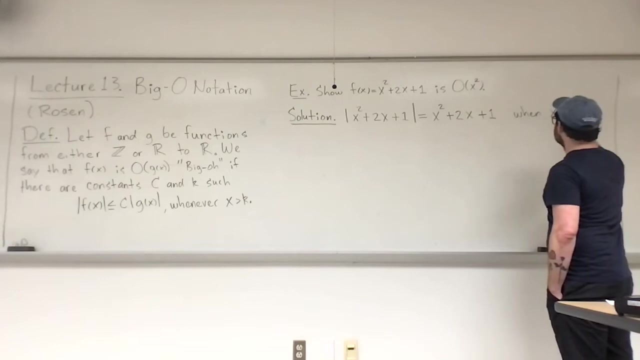 The absolute value of x squared plus 2x plus 1.. Okay, Now it helps to like drop the absolute values, Okay, When kind of manipulating sums and stuff. So I'm just going to note that this is like equal to x squared plus 2x plus 1 when x is greater than or equal to 0.. 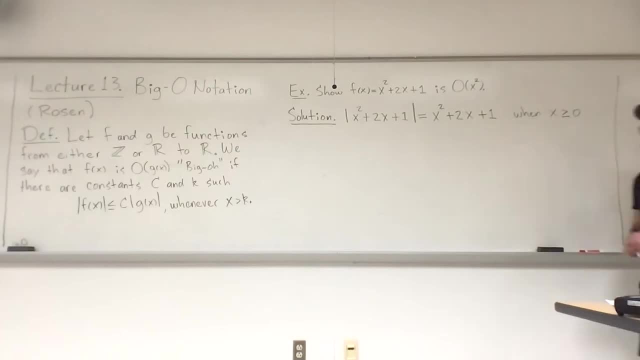 I can just drop the absolute values, right. Okay, In fact, when like that part's like greater than negative 1, it's going to be positive, right, And you drop the absolute values. But this for sure makes me can drop the absolute values right. 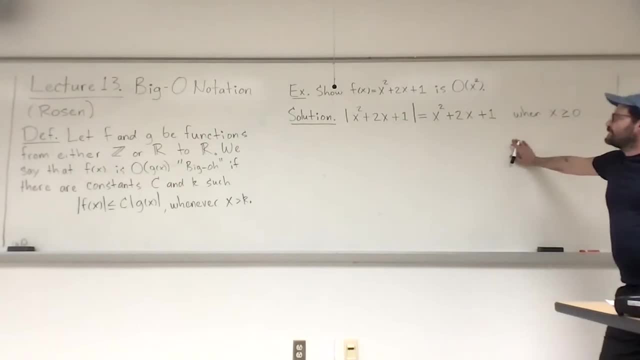 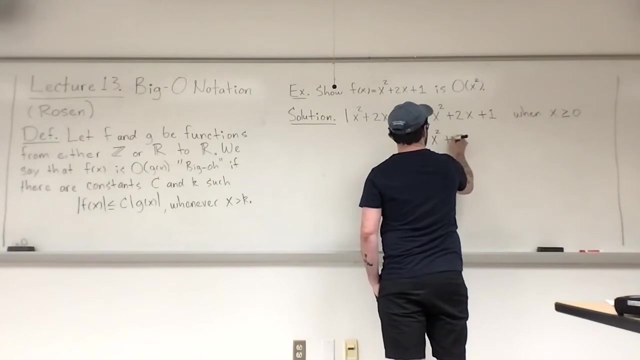 So then I have to think about like: okay, My goal is to get to like some constant multiple of x squared right. So next, observe that this is at most x squared plus 2x plus 1.. 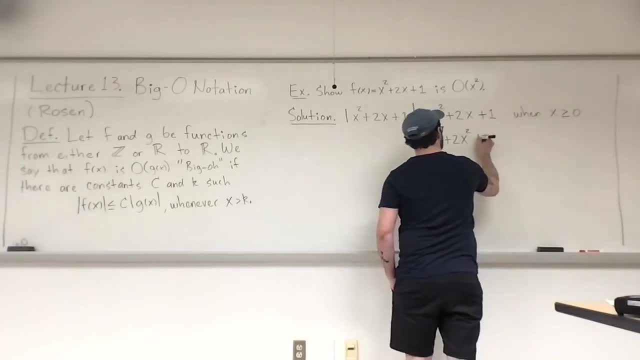 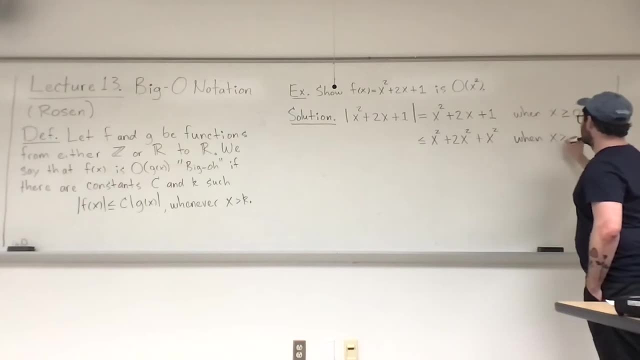 Okay, Plus 2x squared, plus x squared when x is greater than or equal to 1.. Why is that? Because x squared is greater than or equal to x when x is greater than or equal to 1.. Right, And if x is greater than or equal to 1, then x squared is also greater than or equal to that 1, right there. 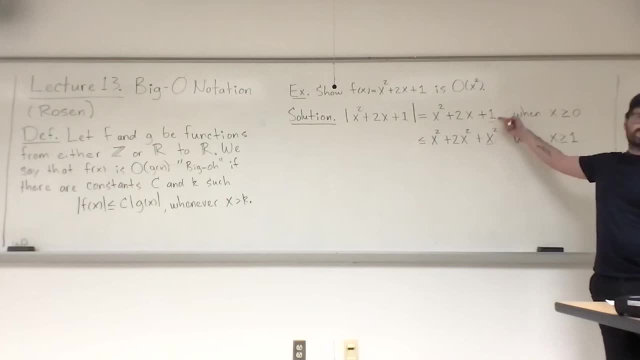 So like that and that, So that's greater than or equal to that, And then that is greater than or equal to that. It's important that x is greater than or equal to 1, though, Because if x was in the interval 0, 1,, then the square is less than x. 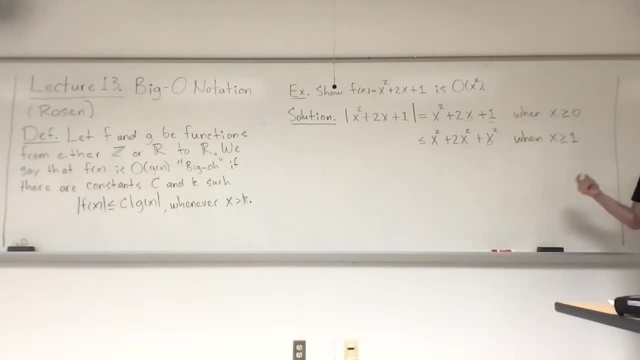 I think about like 1 half squared is 1. fourth It gets smaller, But if it's greater than or equal to 1, then I know that's greater than or equal to that. That's greater than or equal to that. 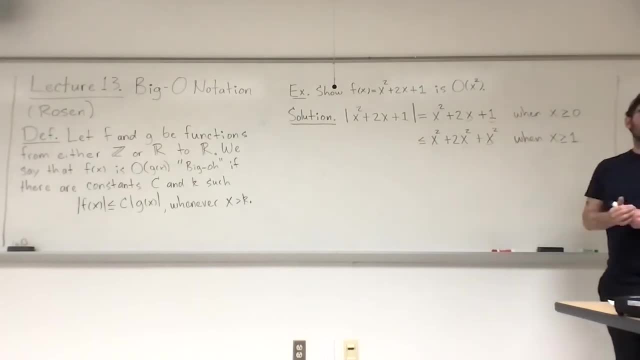 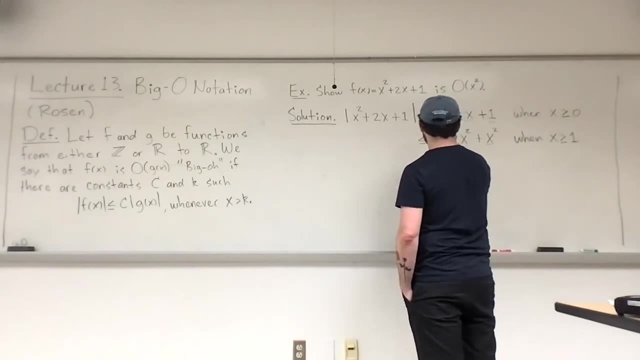 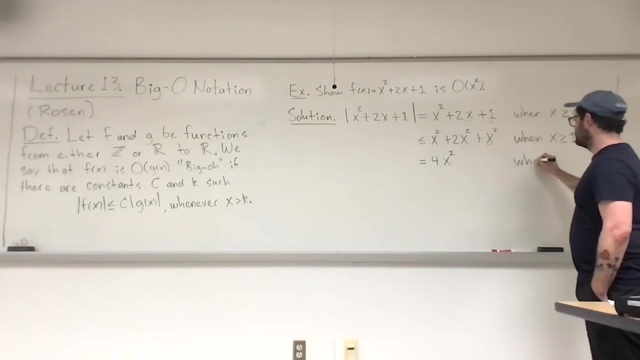 Okay, So then I just have like terms. I can combine them Right. So this is going to be equal to or x squared, And again I'm keeping track of my condition on x. Okay, So now this is the same thing as writing. 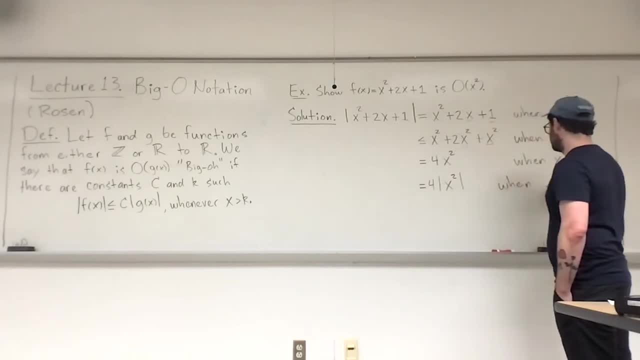 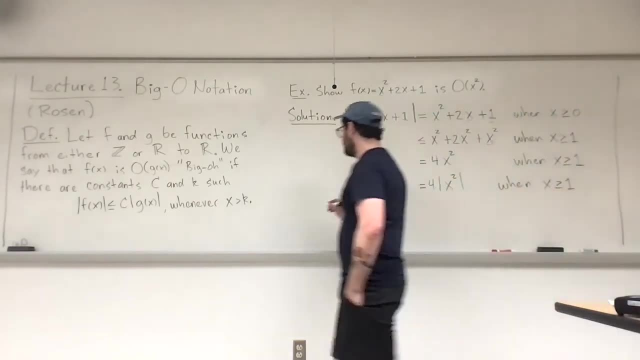 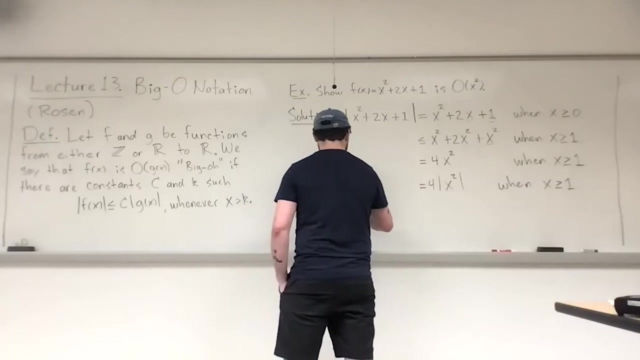 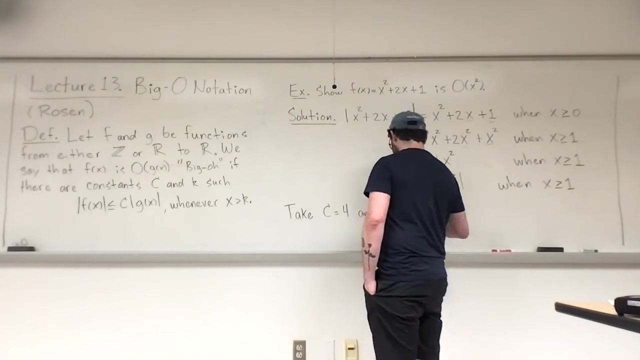 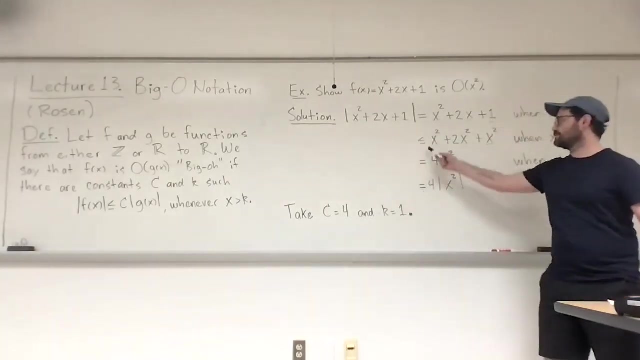 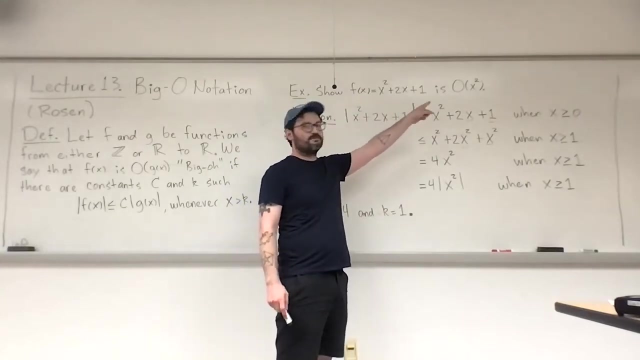 So this is going to be equal to or equal to x squared. Okay, function is at most four times the object value of this function whenever x is greater than or equal to one. So basically, what's happening here? is it like this thing gets bounded above by a constant multiple of x squared, kind of quickly? 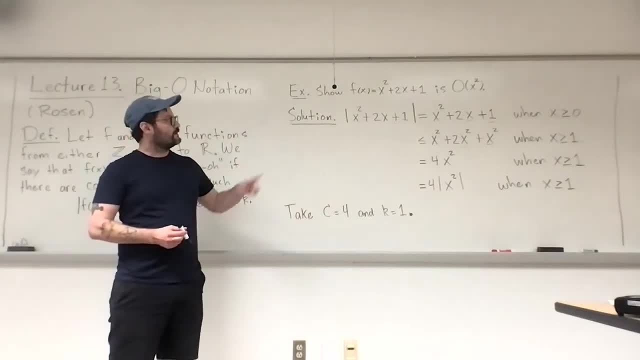 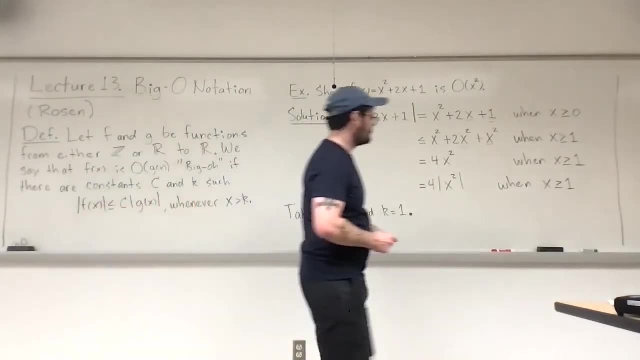 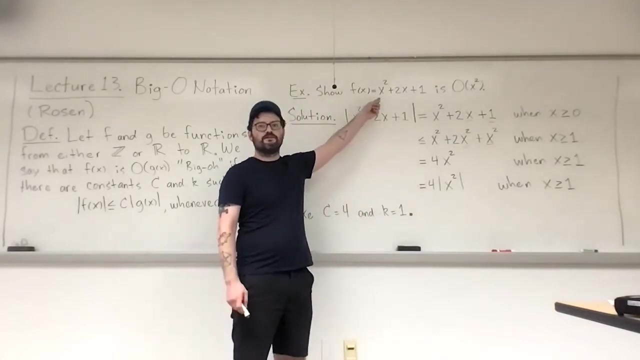 Like, right after x is greater than or equal to one, four times x squared is going to be greater than or equal to that function. So it's just a way of like, it's a way of giving a measurement on the growth rate of this thing, this function. 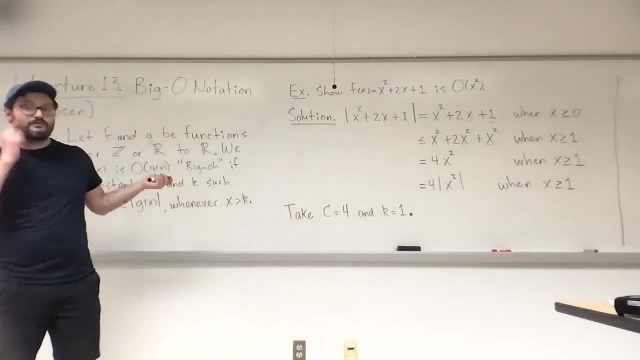 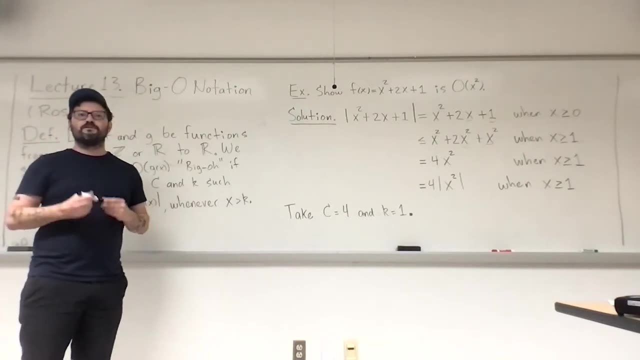 Now, with relation to algorithms like why this, like how this would do it, how would this relate? You can like, given pseudocode, you can measure the number of atomic or basic operations that need to occur, Like: how many times? 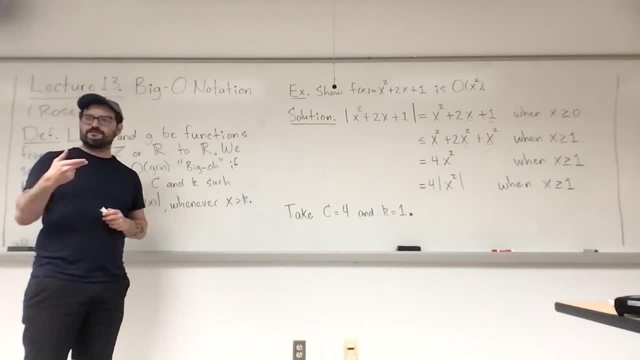 how many times that you're like adding something, how many times you're checking a boolean statement. You can count the number of operations in an algorithm and write it as a function. It'll probably be a messy function, but then you want to kind of give a measurement to that. 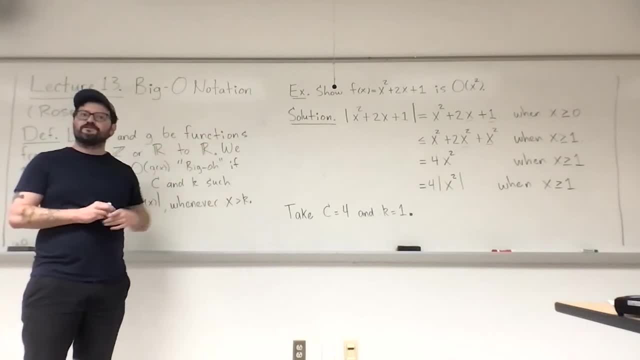 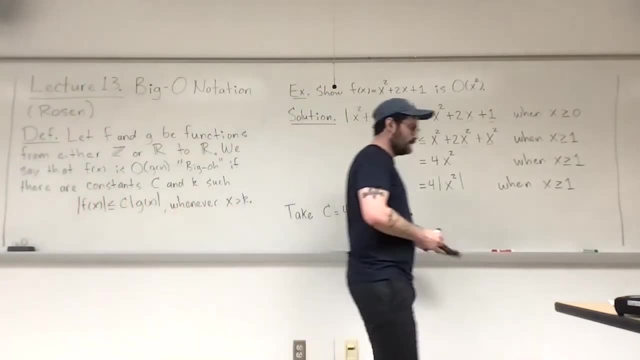 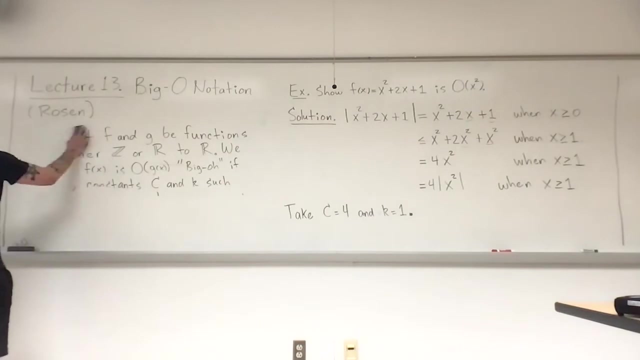 function. It's big O of some simple function. So it's like a way of measuring how complex your algorithm is. So that's like where we're going. Okay, So let's look at another example. This is the just happensIsn't that that doesn't work. 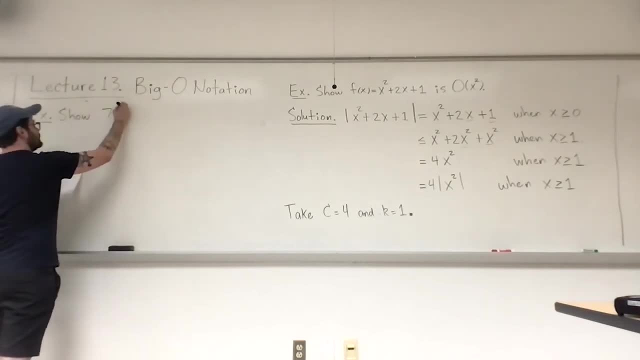 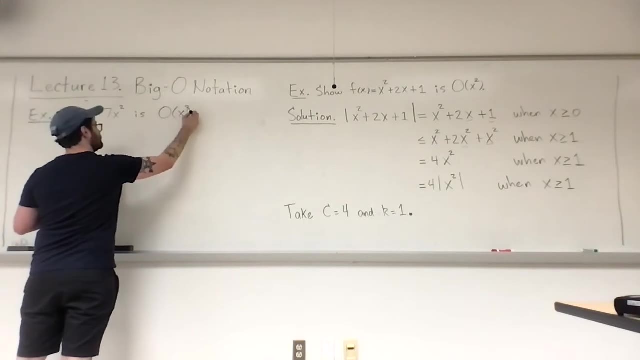 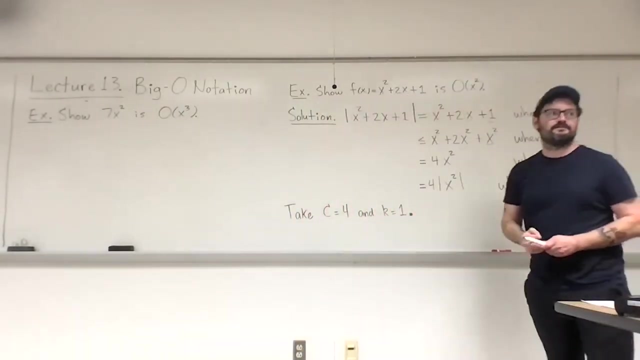 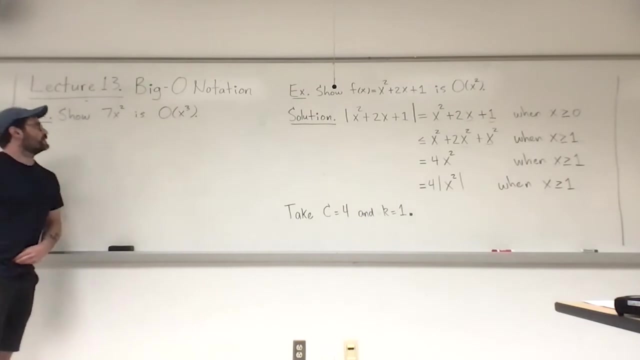 Okay So. so Now this one is like almost like easier in a sense, because they, as soon as like X is greater than or equal to seven, this is going to be, at most, X times X squared, which is execute right. so this one is like kind of easier, which is still right off the formal solution. 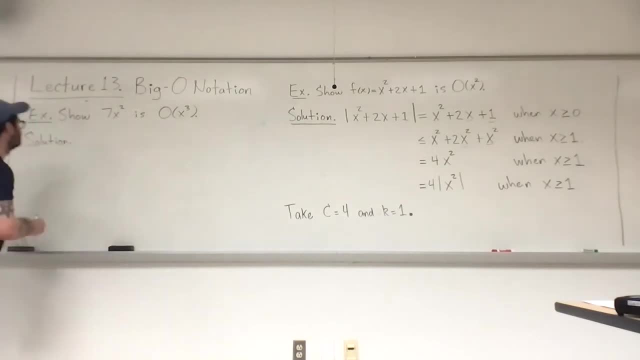 So just look at the absolute value That This is equal to seven X squared. That's always positive in there. We don't have any conditions on X, It's just positive, Okay. And then this is at most X times X squared is another way of writing right over there. 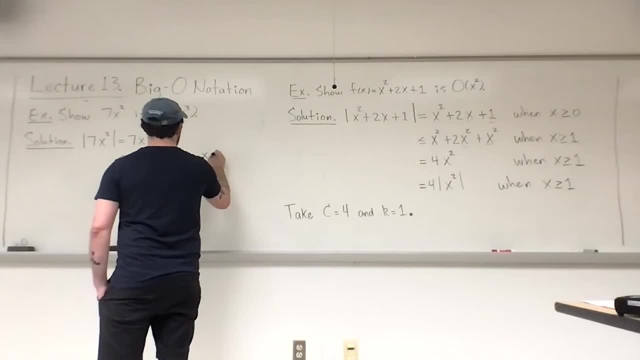 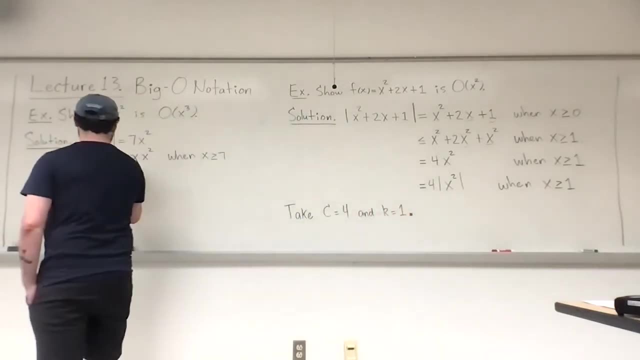 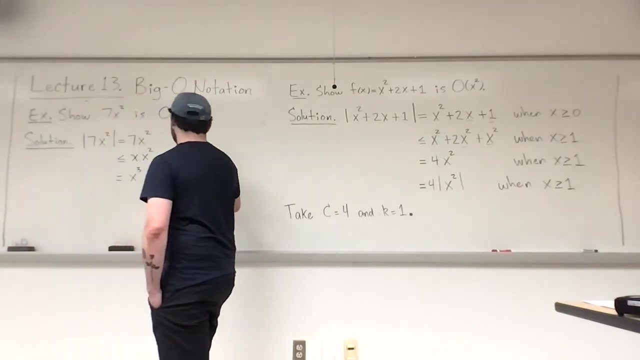 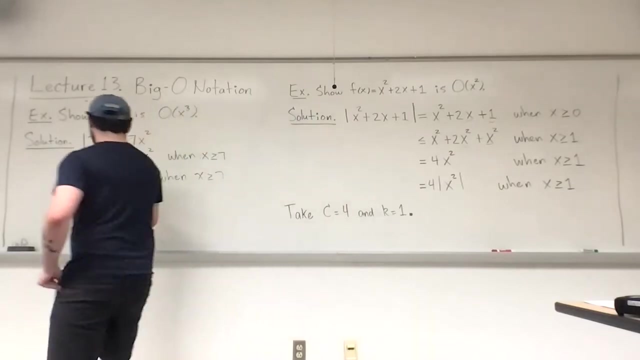 Whenever X is greater than or equal to seven, This is equal to X cubed, And I'm just like you don't really have to do this. I just like to keep track about this business here on each line personally. And then finally, 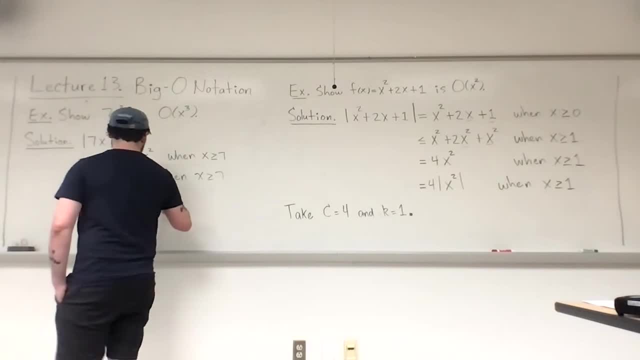 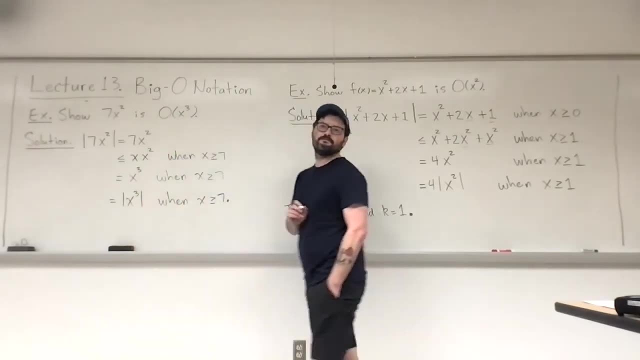 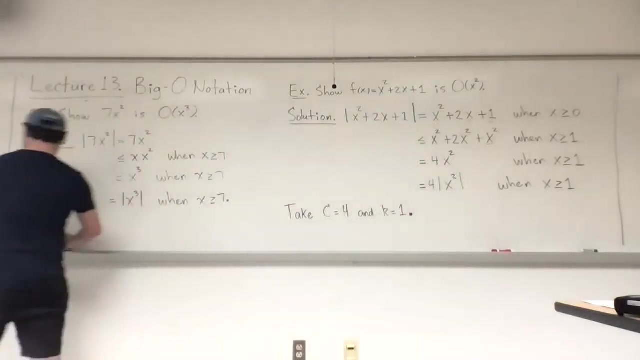 This is equal to the absolute value of X. cubed Again, X is greater than or equal to seven. So we found our C and our K. C is one, K is seven. These are called the witnesses to the big O instance. 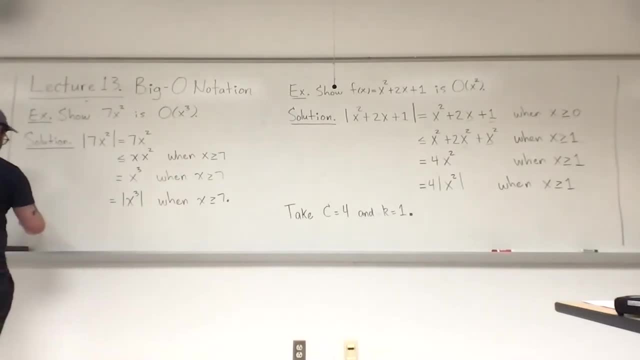 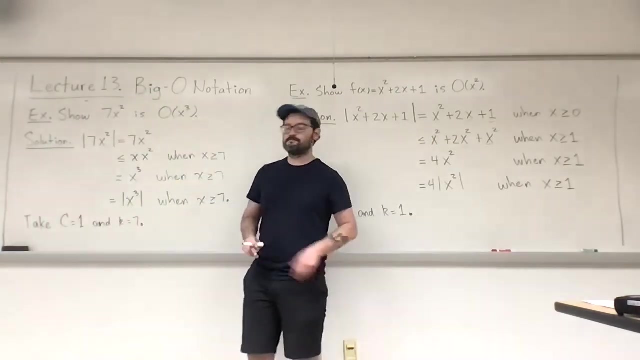 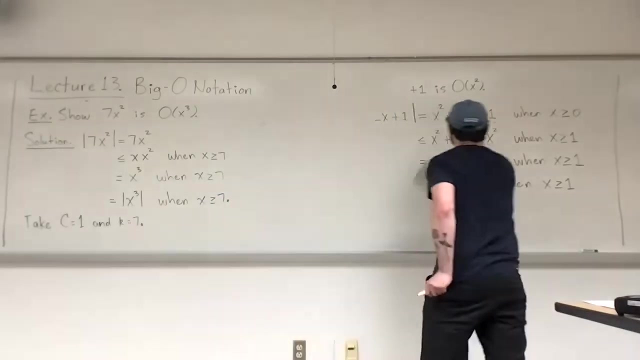 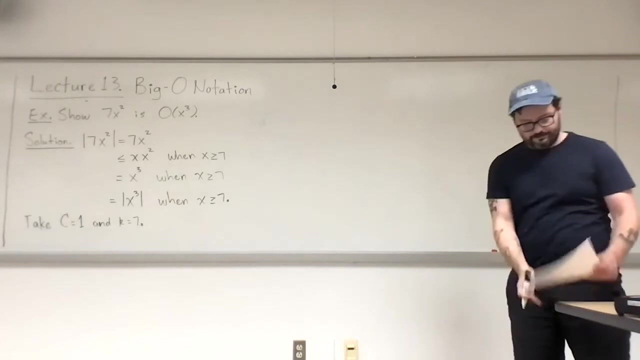 So then you would just write this explicitly out: Take capital C equal to one And lowercase K is to be seven. Now Now Let's look at a case where we show that a function is not big O of another one. So 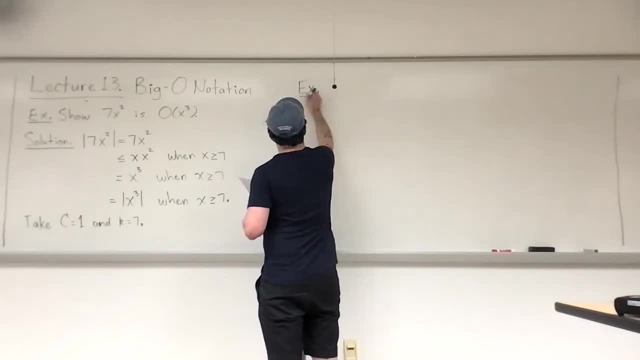 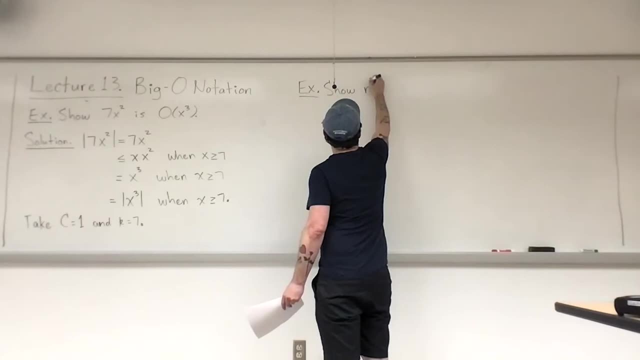 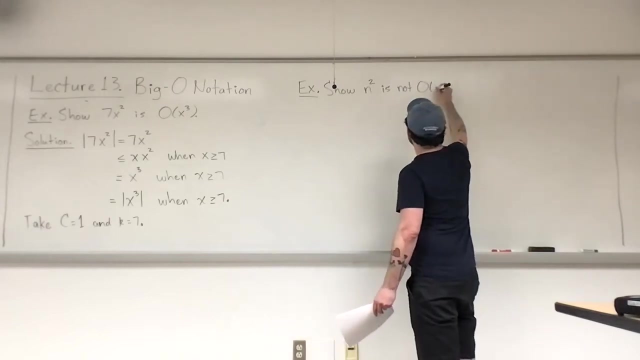 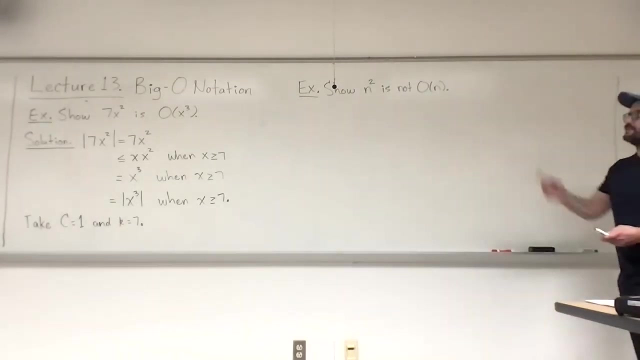 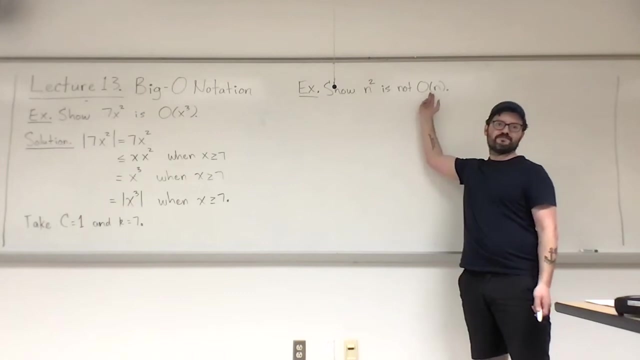 So, So, N squared is not big O of N. Now, Sure, This one would make immediate sense that that's not big O of N. Right, Like There's no constant that's going to save this, Like, Like. 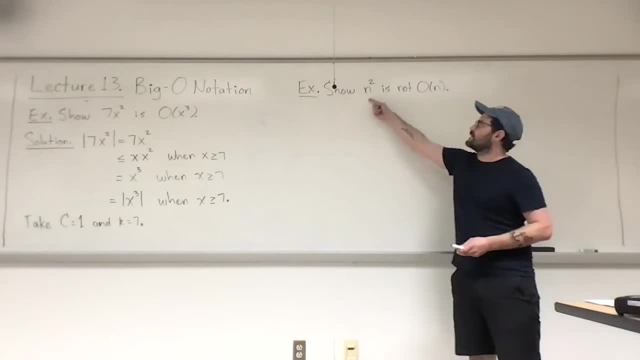 Not falling behind that Right, Because this is like N times N, Any constant times N. As soon as N is larger than that constant, then that's going to be bigger Right, And that actually points to like how you would show this. 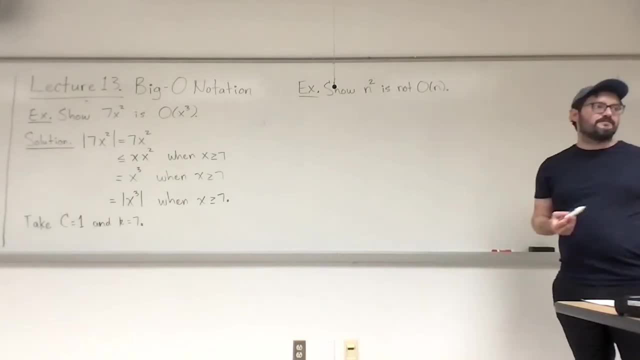 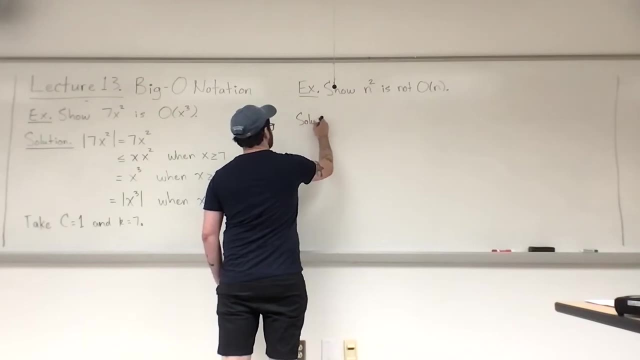 You would assume by contradiction that it is big O And then get a fallacy So So. So If you're going to show something is not big O of another function, then the way to do this is with contradiction, pretty much every single time. 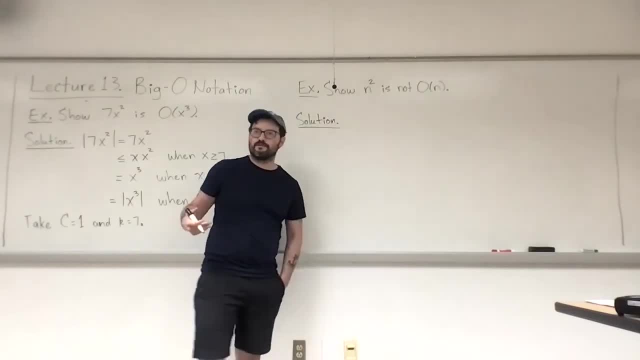 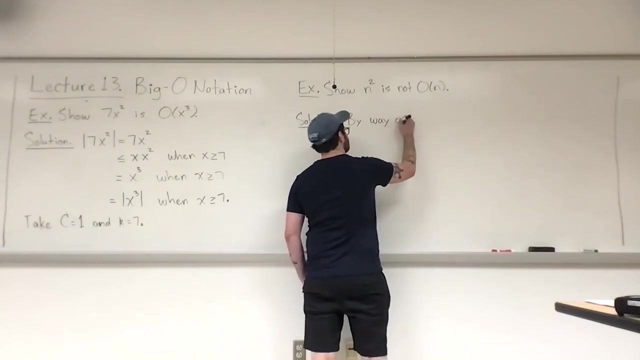 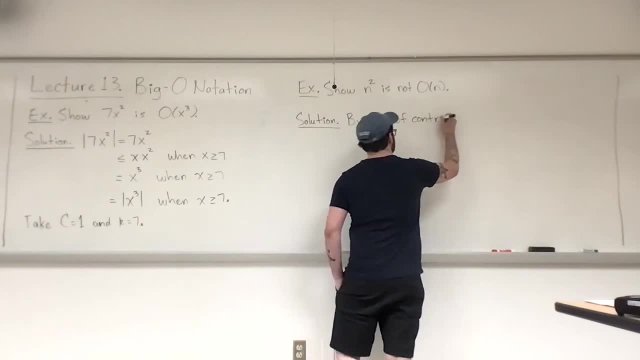 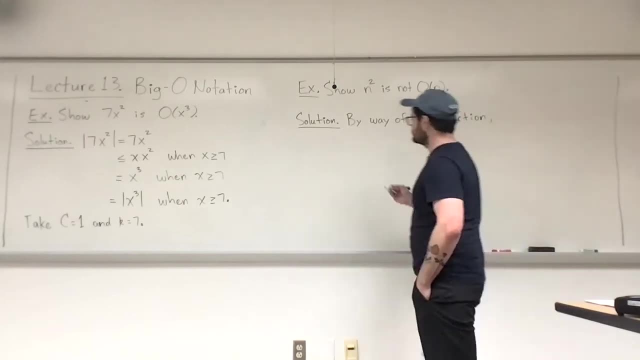 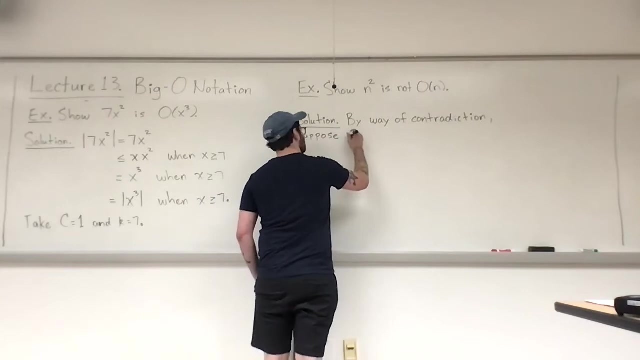 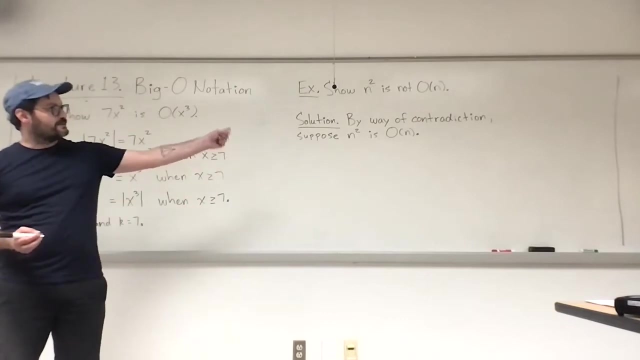 So, So, So, So. Now last thing about contradiction is that under this assumption we get all this information. We get that there's witnesses to that big O instance. So if that is big O of n, then there exists capital C, lowercase k, such as this: 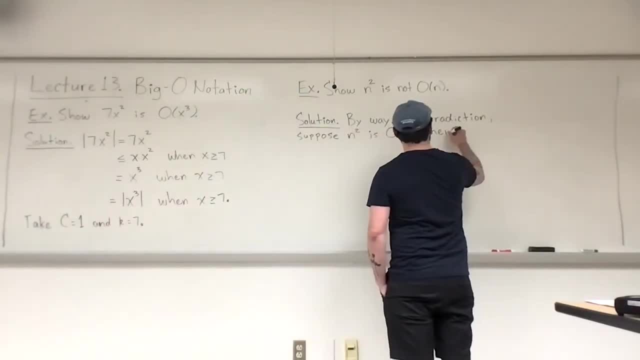 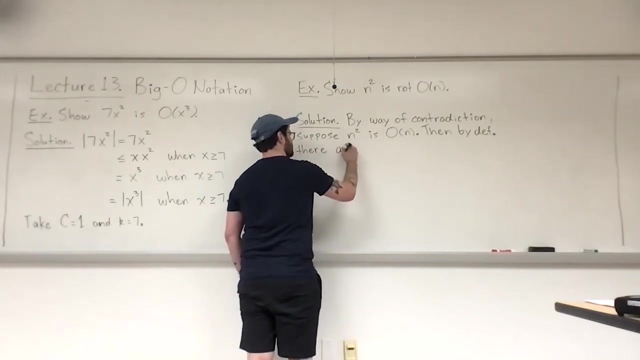 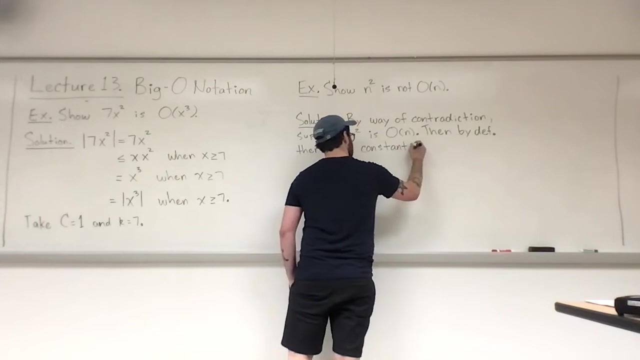 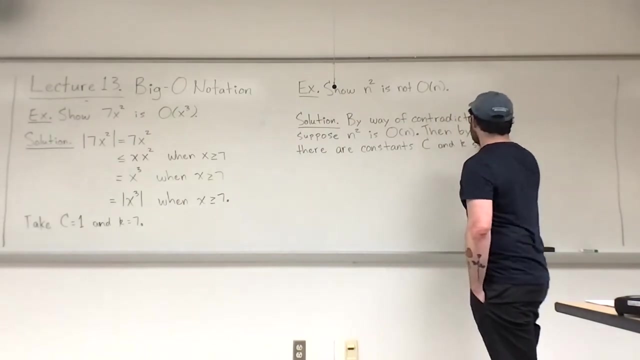 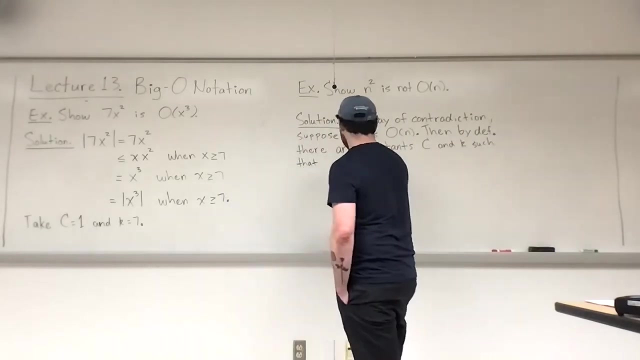 So then, by definition, we'll just write it out. I'll abbreviate definition for the sake of board space. So then, by definition, there are constants, Capital C and lowercase k, such that the absolute value of n squared is, at most, C times the absolute value of n. 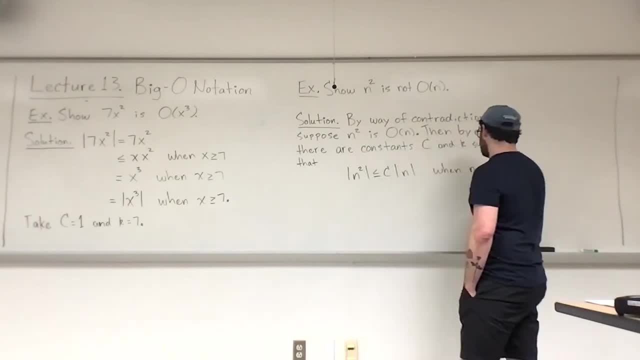 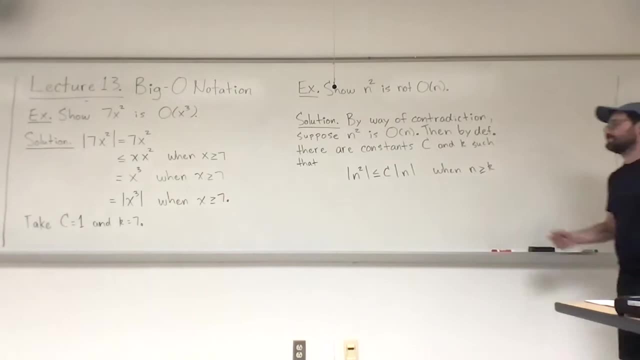 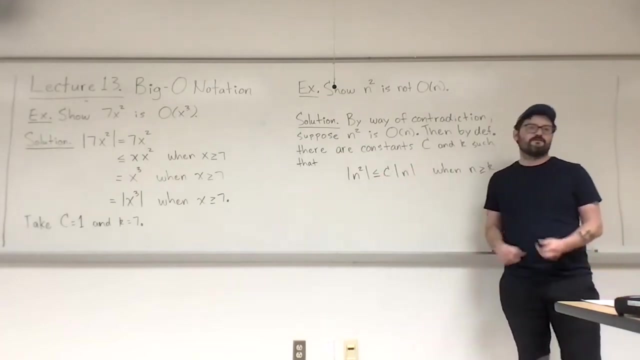 When n is greater than or equal to k. So this is for any n greater than or equal to k, right Any n. So eventually, like n is going to be positive, right, At some point n has to be positive, which means we can drop the absolute values. 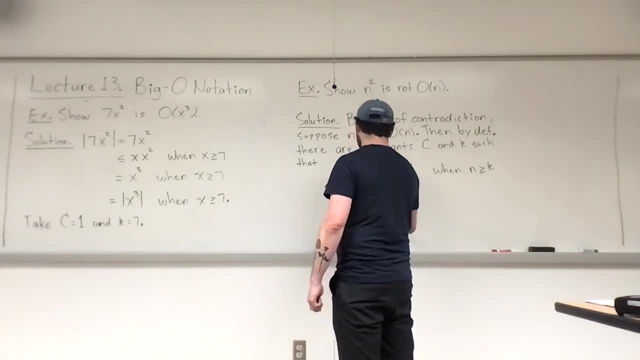 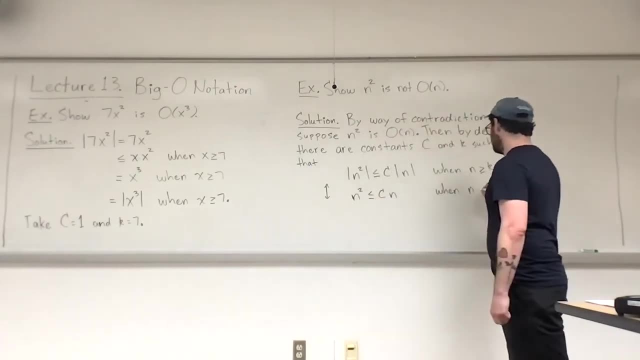 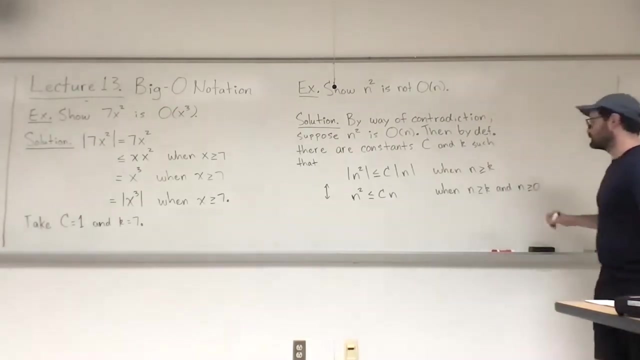 So this means So when n is greater than or equal to k and n greater than zero or equal to zero, whatever, Okay, And then, since n is positive, right, we can divide both sides of that inequality by n. 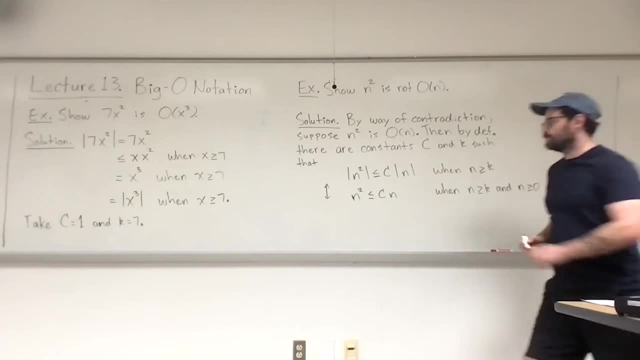 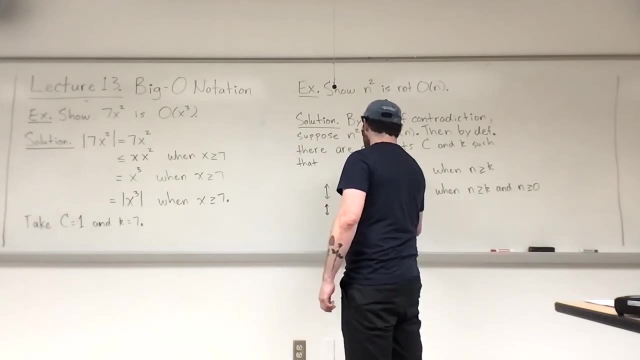 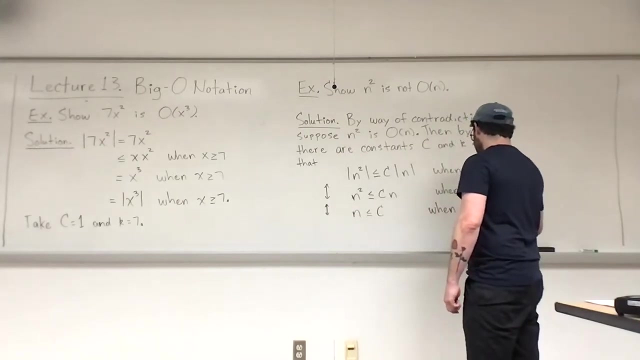 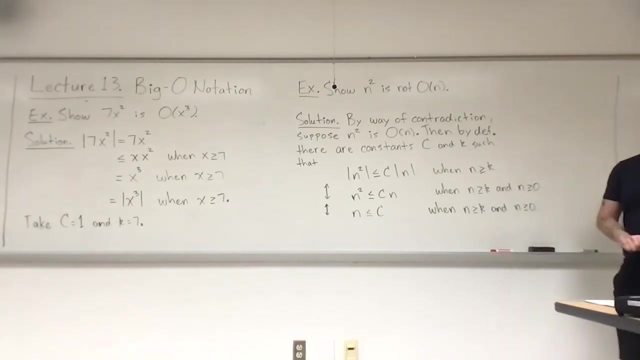 And the inequality Doesn't change direction or anything. So we get that n At most C, And again when n is greater than or equal to k and n is greater than or equal to zero. So for any n that satisfies this, that's going to be true. 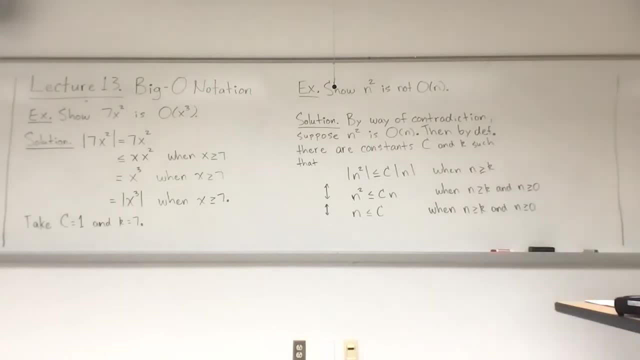 What's wrong with that statement right there? What's wrong with this last line here? Something's wrong, There's a problem. So n is going to keep on getting bigger and what And C is going to stay the same. C is a constant. 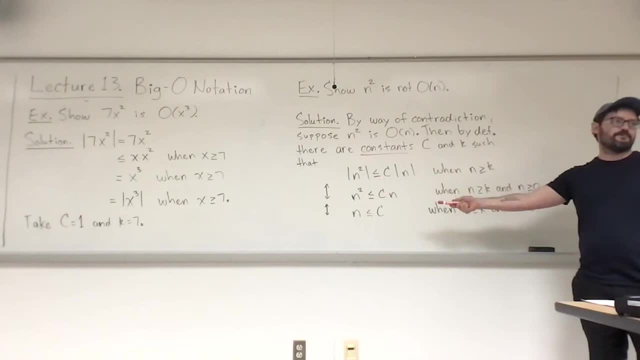 Right, And that's going to fail whenever This has to hold for Every single n greater than or equal to this k right Forever. But C is a constant. So since C is a constant, we need to write that out. 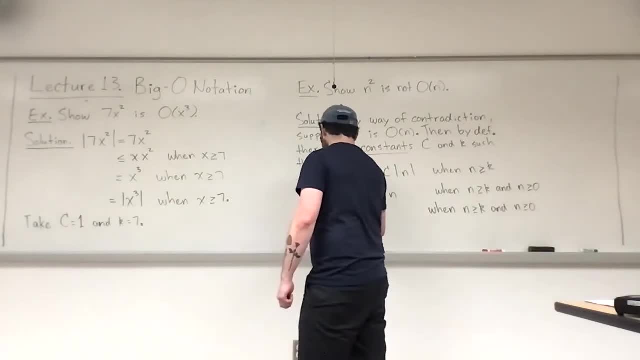 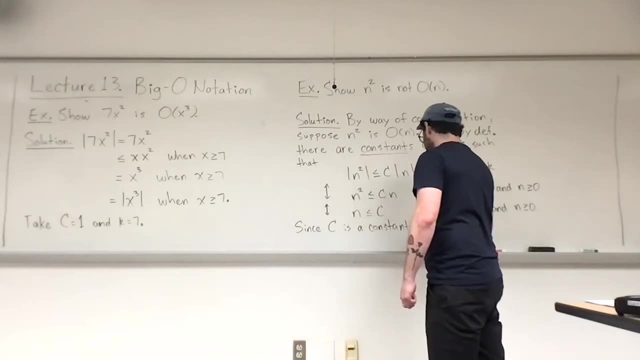 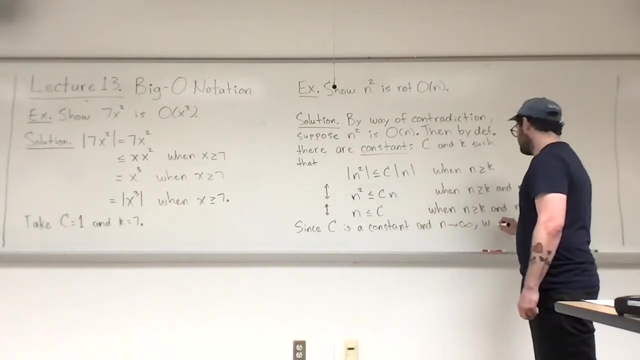 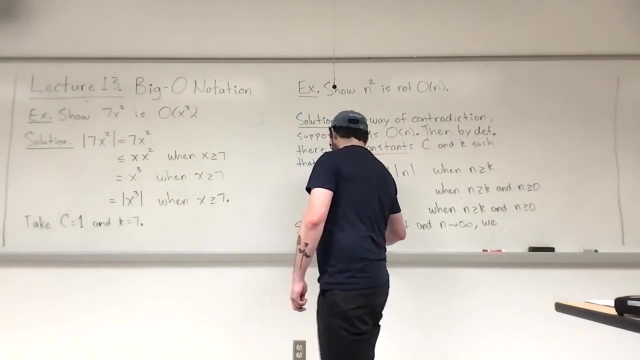 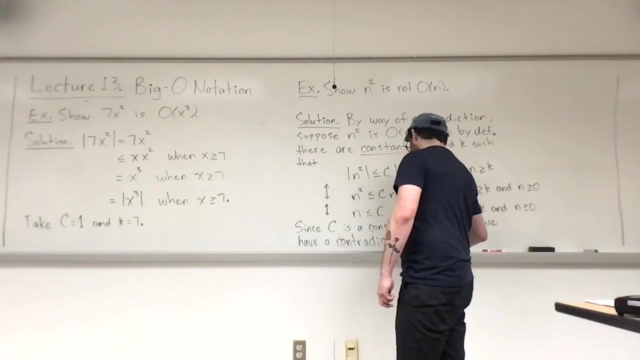 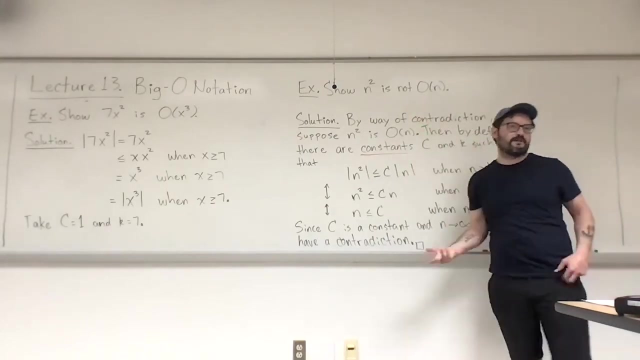 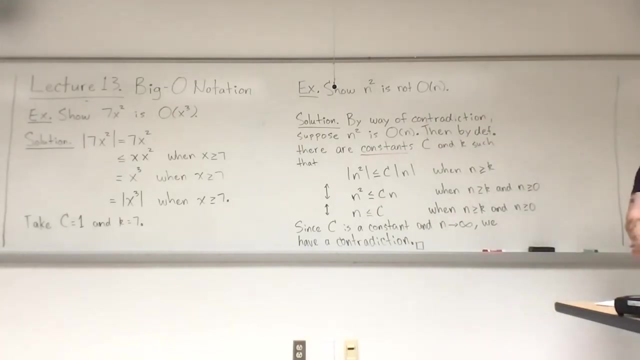 Since C is a constant and n goes to infinity, we have a contradiction. We have a contradiction. It is a proof. So assuming the opposite of this leads to a contradiction. so the original statement must be true. Okay, Any questions about that? 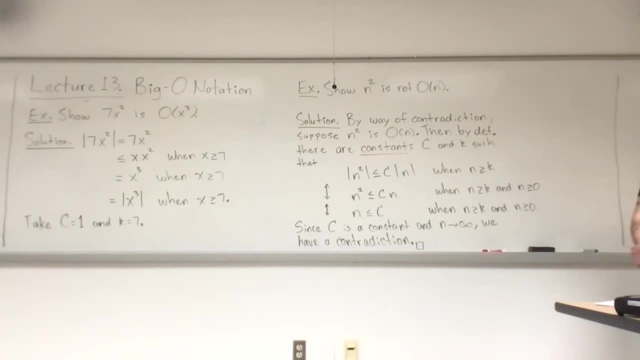 Like, like, like, like, like You could have done it directly now that i'm thinking about it, but I think contradiction also, it's just easier Alright. so there are some important theories and like, like they go results on, like these, like base functions, like all no meals, logs, exponentials, things like that, and that's what we're going to kind of drive next. 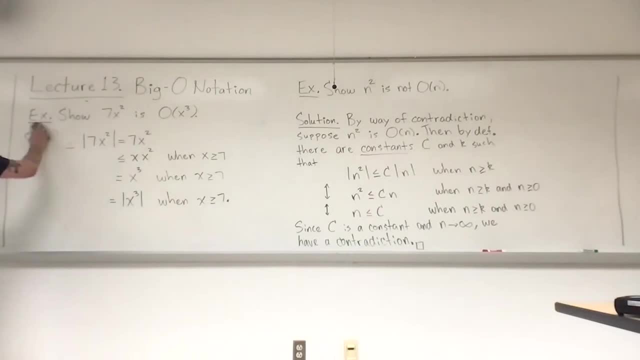 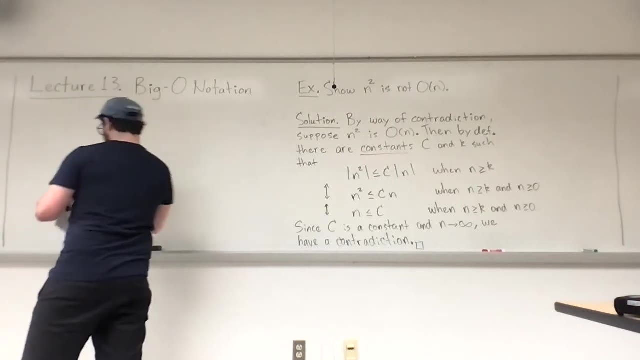 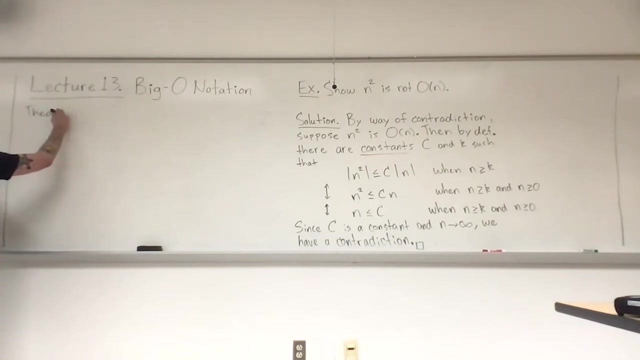 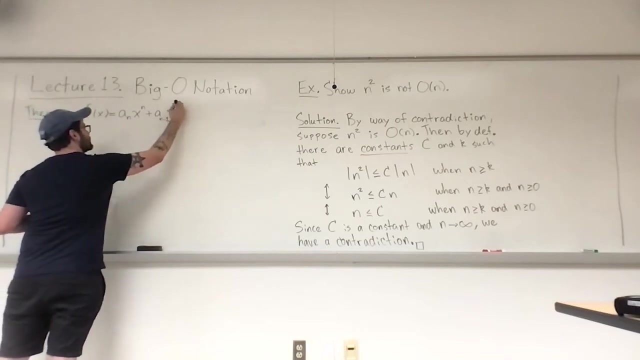 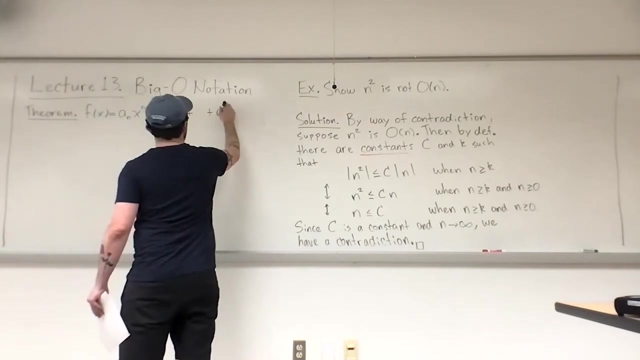 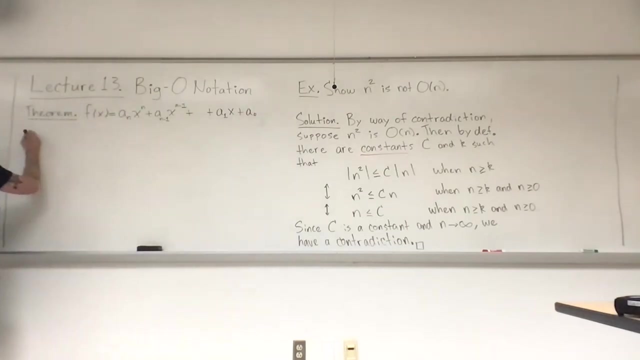 We're going to start with the theorem, general theorem about polynomials. So So f of x equals two Base A subscript n times x to the power n plus a subscript n minus one times x to the power n minus one plus dot, dot, dot plus a one times x plus a zero is big O of x to the power n. 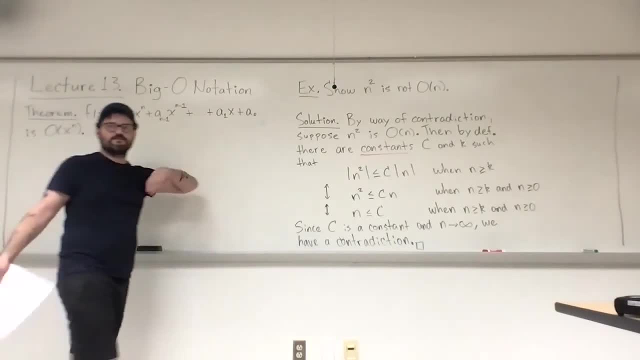 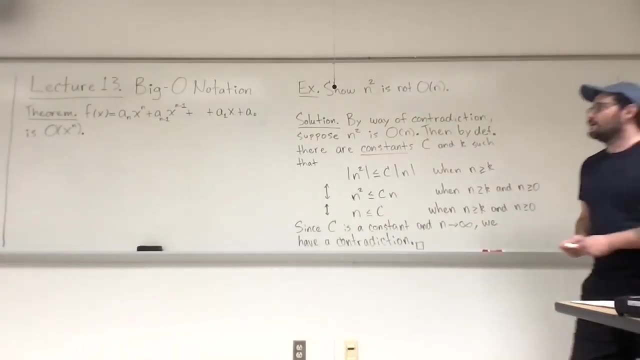 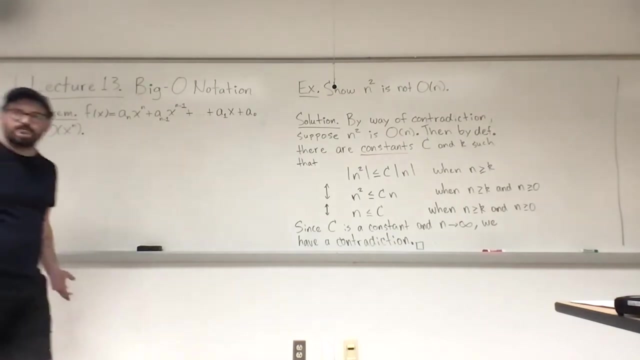 Okay, I hope we recognize this, this notation here. This is a polynomial, So all those days are real numbers. A in is non zero, It's a polynomial. So basically this is saying that if you have a polynomial degree n, then that function is big O of x to the power n, which is kind of related back to, like what we said earlier. 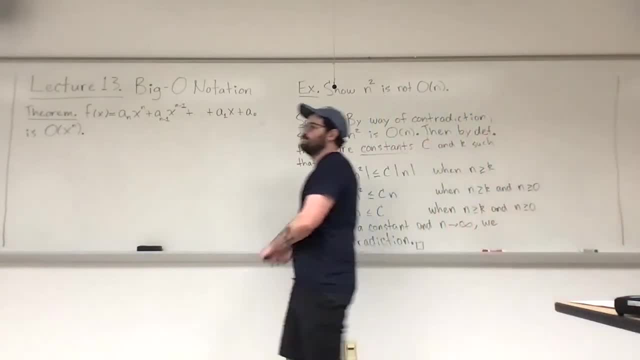 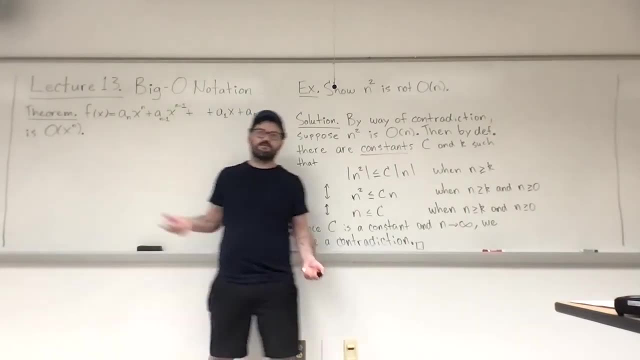 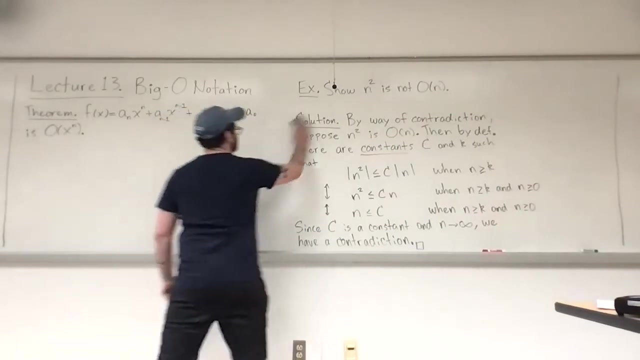 Right, Like when x is huge right. The next is like: two to the power. A trillion Like this means nothing compared to that. It means absolutely nothing, And that's what's like dominating that, that term. Okay, Now to write off the solutions of this. we need a lima. 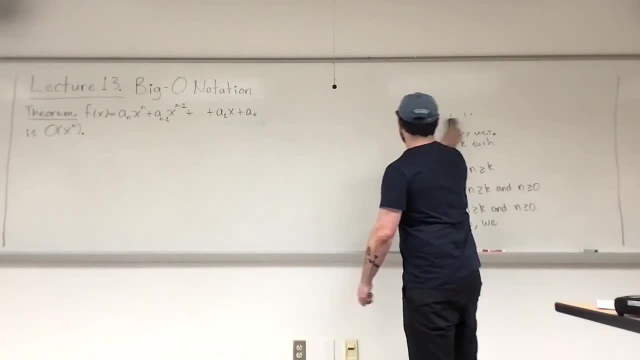 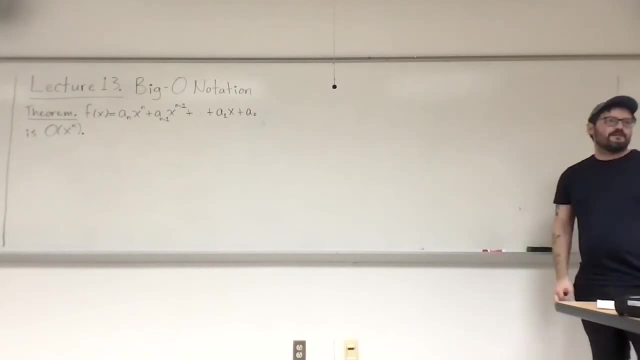 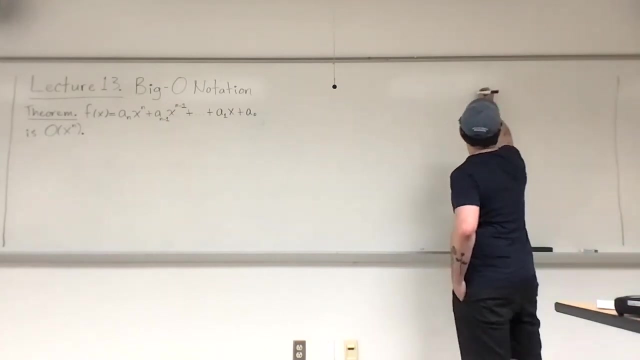 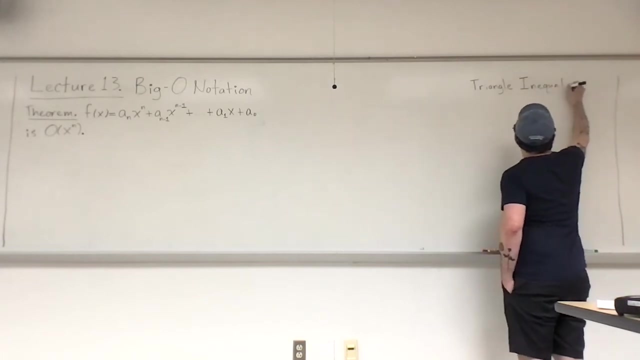 You know, lima, Derived from the Latin word Roughly translates to A tool. It's a, it's like a proposition or a theorem. It is used as a tool when proving other things And it's called the triangle In quality. 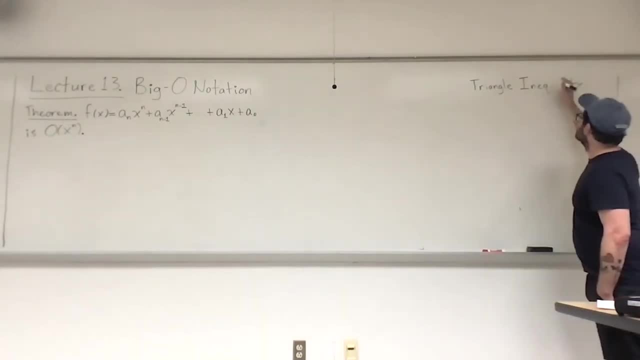 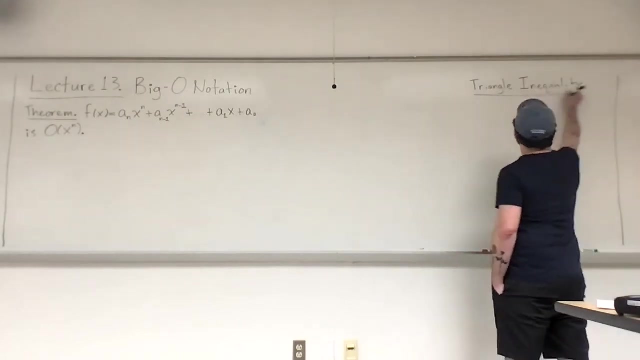 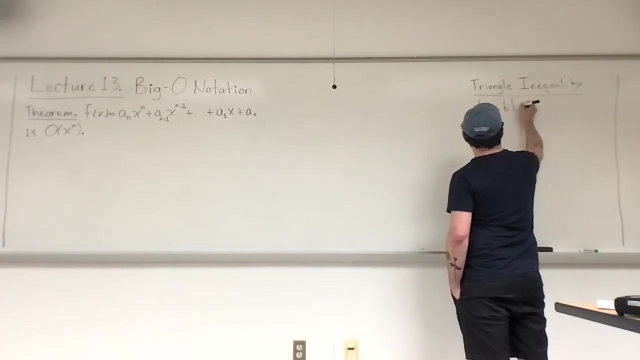 Okay. So have any of you ever heard of the triangle in quality? So it basically states- in its most basic form It says this- That the absolute value A plus B Is at most The sum of the absolute values. That's like the most. 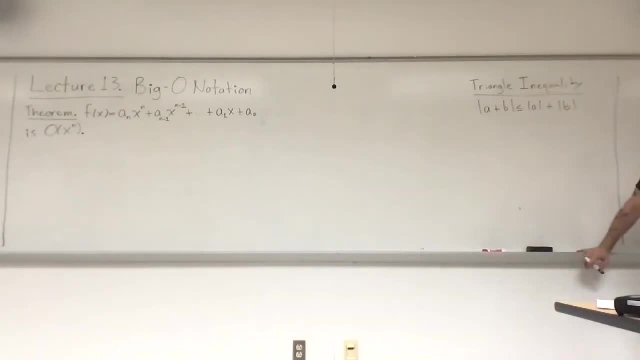 Commonly used form, But this extends to any number of things. So, like the general version, is this So: X1. Plus X2. Plus Dot dot dot Plus XN, And absolute value Is at most: 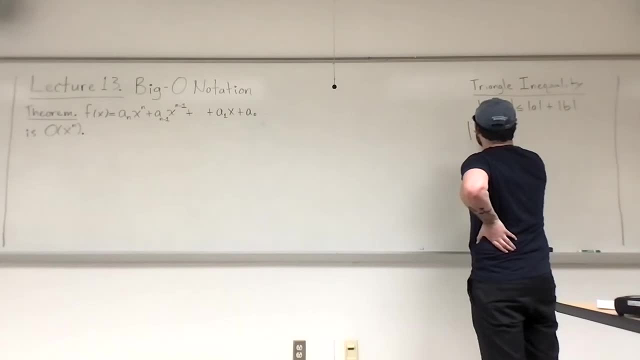 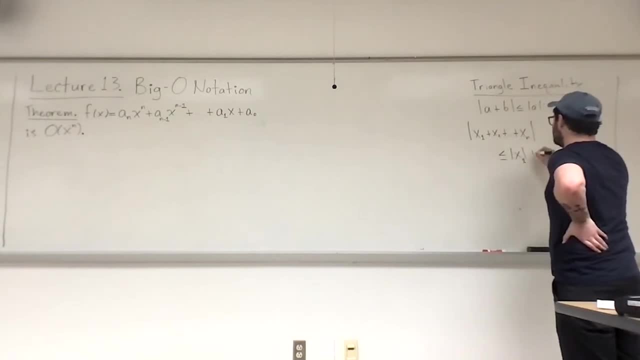 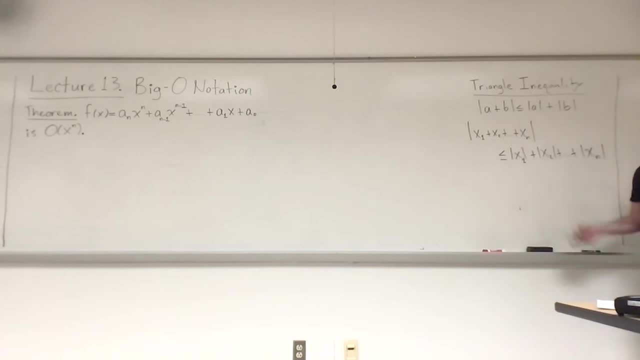 Plus dot, dot, dot Plus. Absolute value of XN. That's the general version When N is 2. It's like the same Right. So The absolute value Of the sum Is at most The sum. 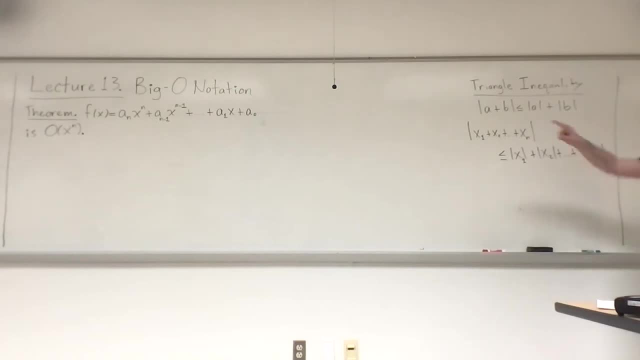 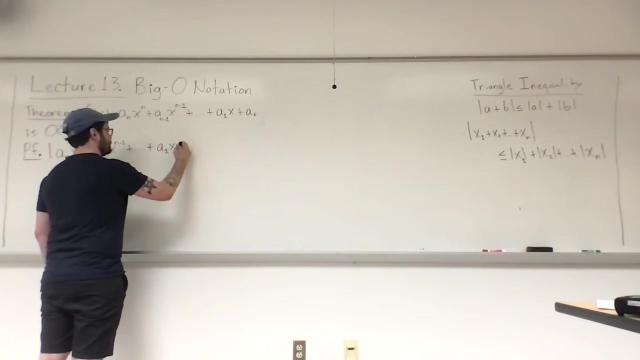 Of the absolute Values Or any real numbers. Ok, And we're going to Use that Over here. Okay, So I'm going to start by looking at the absolute value of this polynomial. nought big O absolute value. 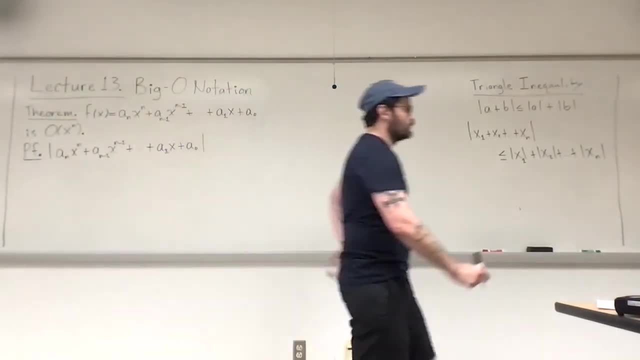 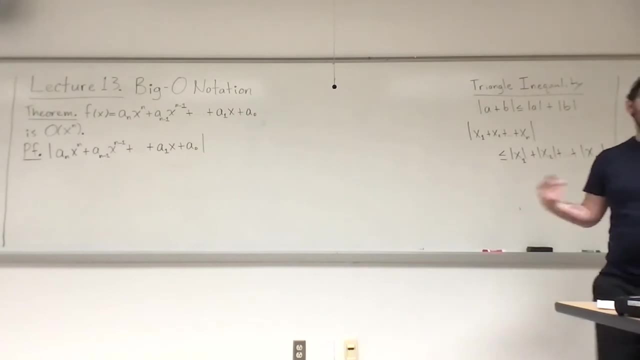 Okay, And then we're going to immediately apply the generalized triangle involved We will have: the absolute value of the sum is at most the sum of the absolute values, Right? so absolute value of nought is at most the sum of the absolute values. 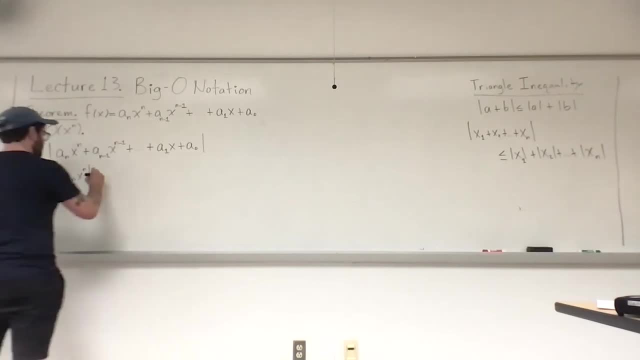 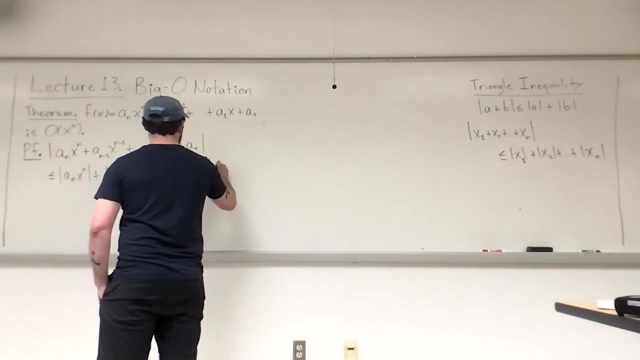 Okay, a n times x to the power n plus the absolute value of a. n minus 1 times x to the power of n minus 1 plus dot dot dot plus the absolute value of a. 1 times x plus the absolute value of a naught. 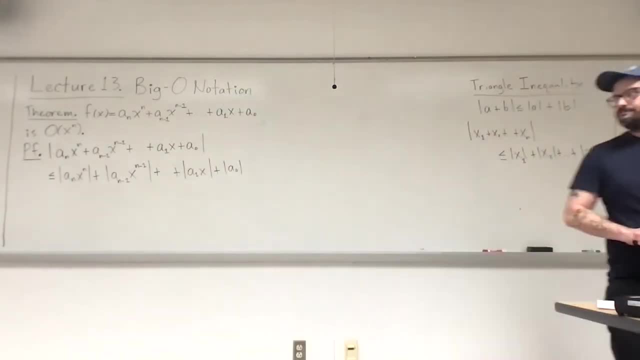 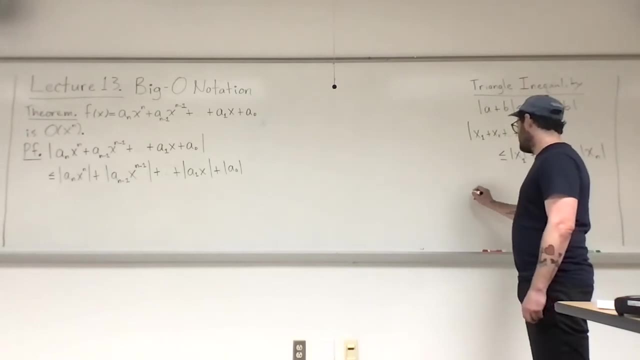 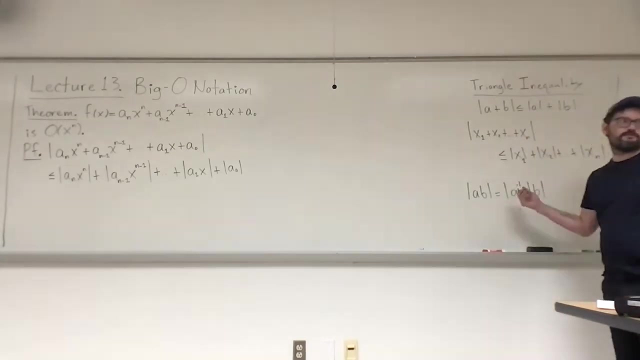 And that's by the triangle: inequality. Okay Now, so this is like an inequality. a property of absolute values is this as well: Absolute value of a times b is equal to the absolute value of a times absolute value of b. That's just a property of n equal to the absolute. 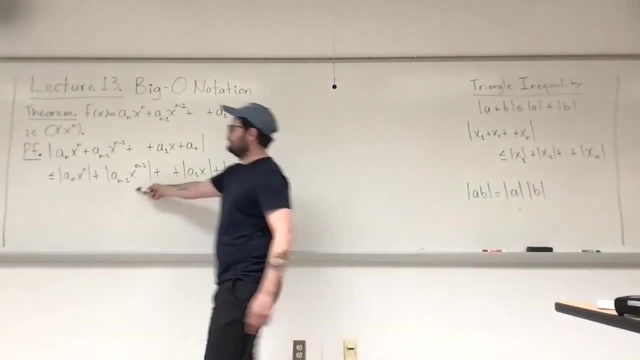 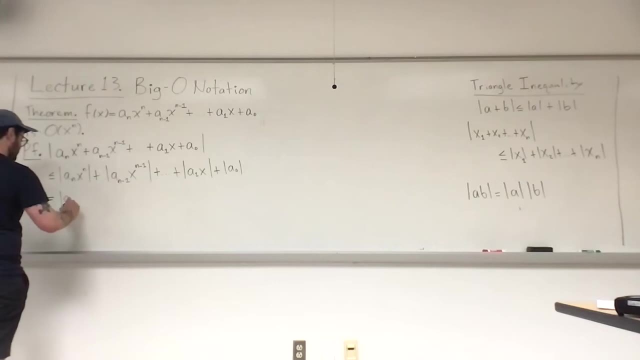 value. So notice, we have like a bunch of like products here, So we can rewrite that So: absolute value of a- n. And I'm going to drop the absolute absolute values on the x, Because I'm just going to assume that x is greater than or equal to 0. 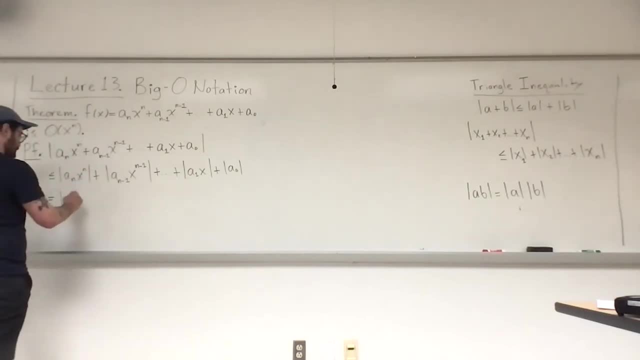 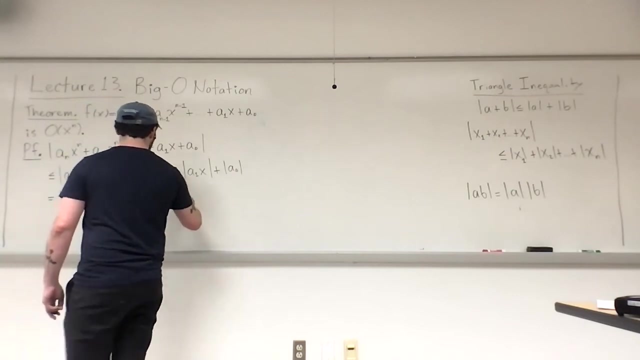 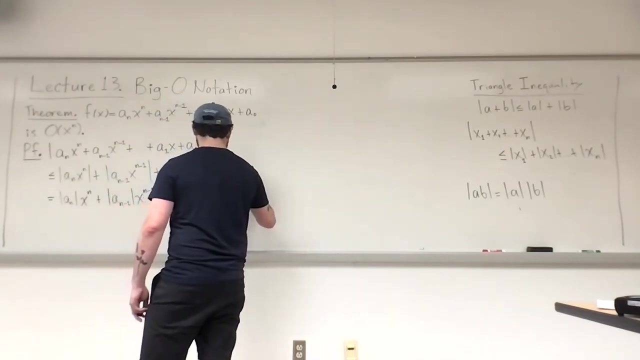 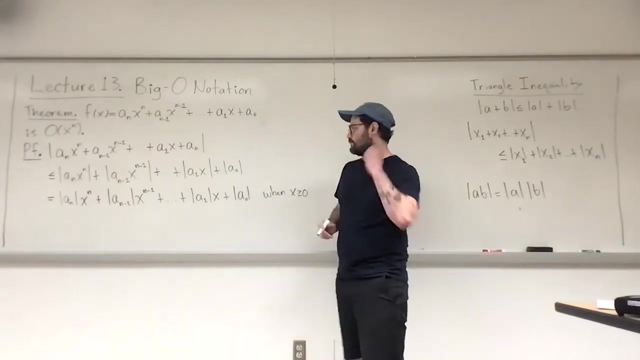 So I can just drop all of those out, right? I have to keep the absolute values with the coefficients though, because I don't know if those are positive or negative. This is when x is greater than or equal to 0. I can drop the absolute values on all those x's. 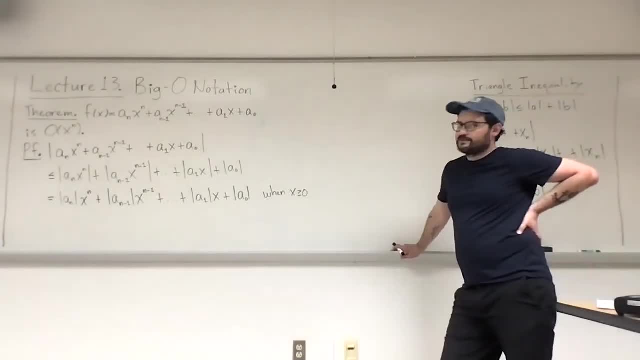 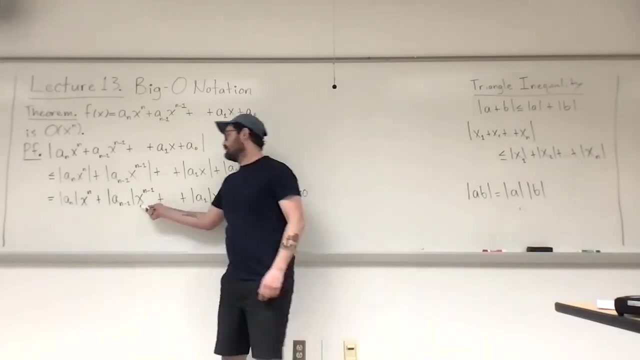 Okay. so next up, we need to somehow write this as a product of x to the power n. So if x is greater than or equal to 1, that's at most x to the power n. That's at most x to the power n. And. 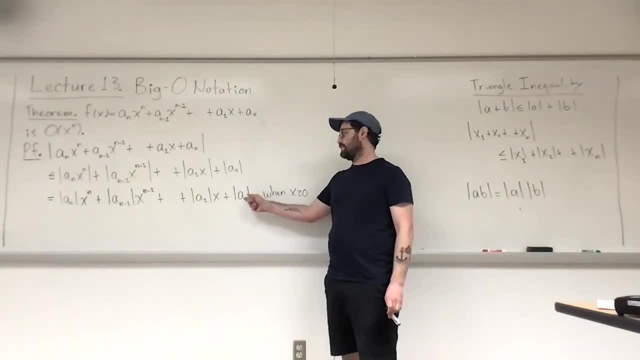 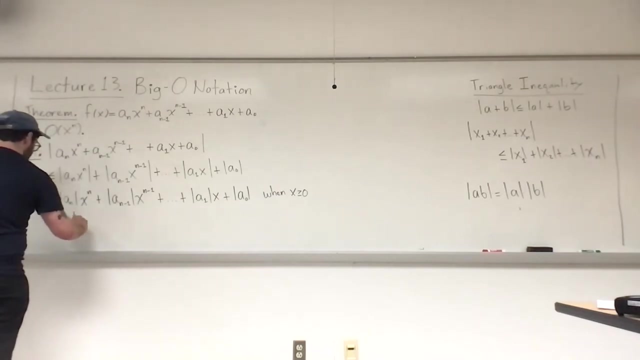 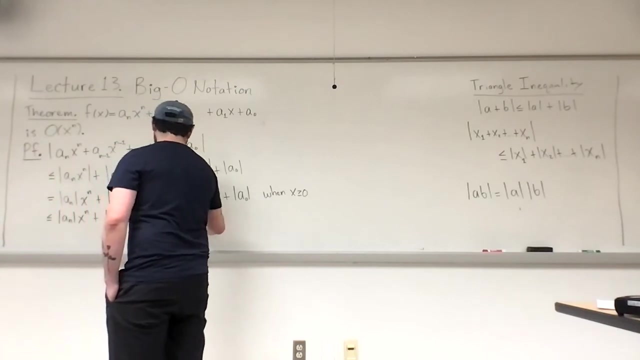 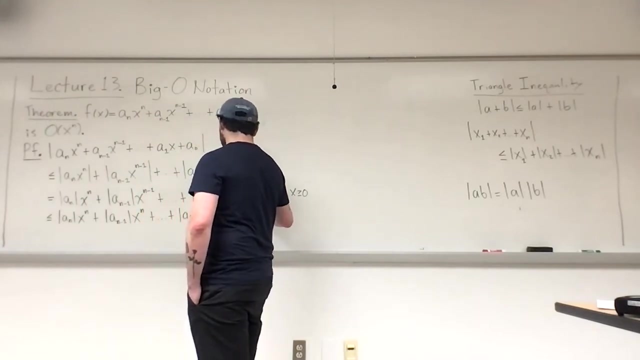 And there's a one multiplying that. right, there's a one multiplying this: a, not a. so if X is greater than or equal to one, X to the power n is greater than or equal to that one. So This is, at most, The absolute value of a n times X to the power n, plus absolute value of a n minus one times X to the power n, plus dot, dot, dot, plus absolute value of a one times X to the power n, plus absolute value of a not times X to the power n. 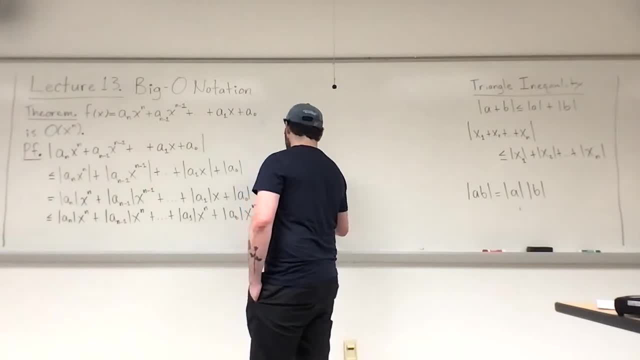 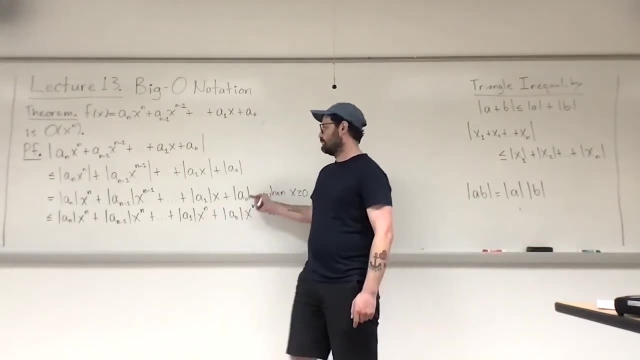 And that's when X is greater than or equal to one. So like: that's great that, that's great that one, that's great that so forth, and so on. right, provided X is greater than or equal to one. Okay, so next. 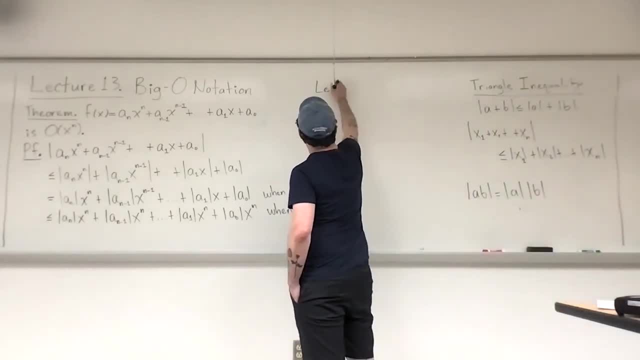 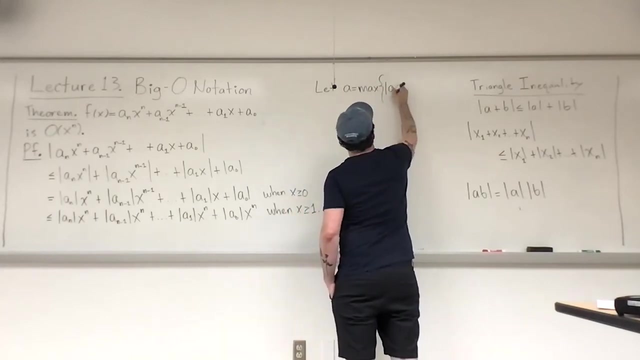 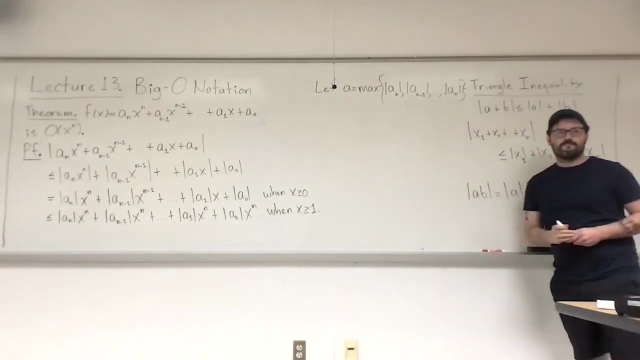 i'd say like: let's A equal to the Max of the sets, As today in common, absolute value day, and minus one comment that that that's absolutely value, they not? So there's a: whenever there's a finite number of things, you can find the maximum. and there is a finite number of things, right, there's in plus one. 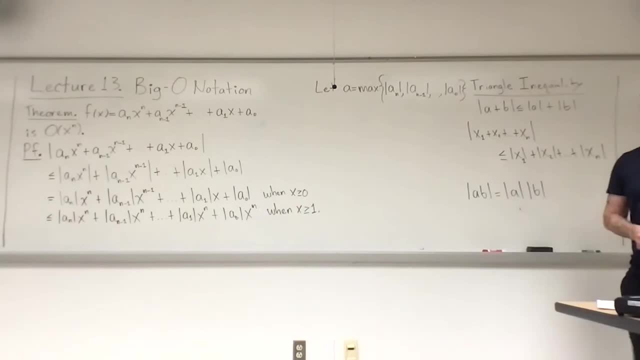 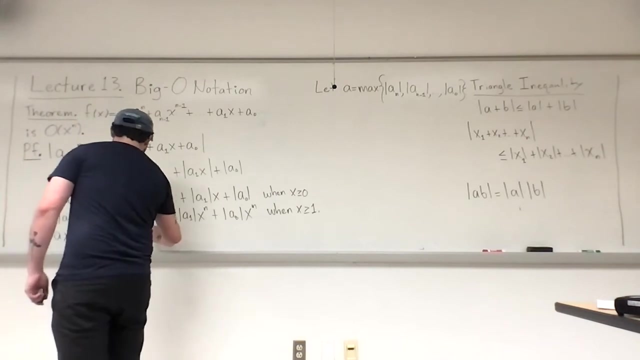 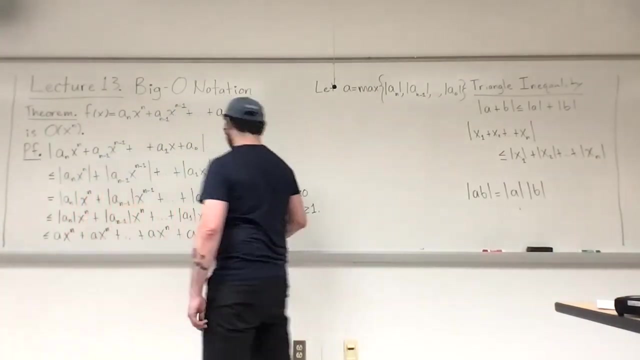 So a is just going to be the maximum all this, So, So, So This year is at most A R? n plus A R n plus A plus R n. i'm not writing the condition on when. 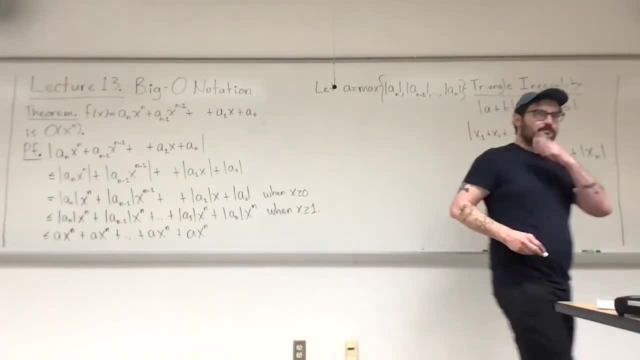 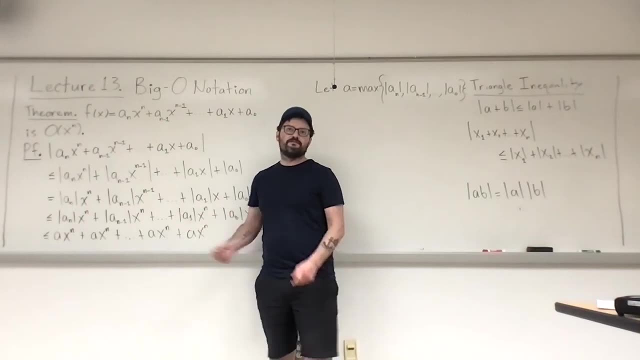 Because i'm going to have to fit stuff This way now. But you see that, right, like a is the largest of all the coefficients and magnitude, so this is definitely greater than or equal to this. How many of those do we have? 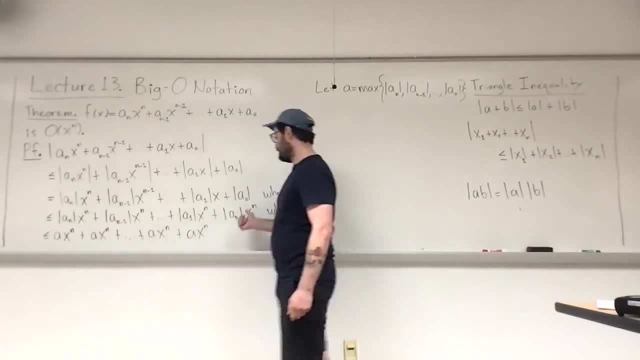 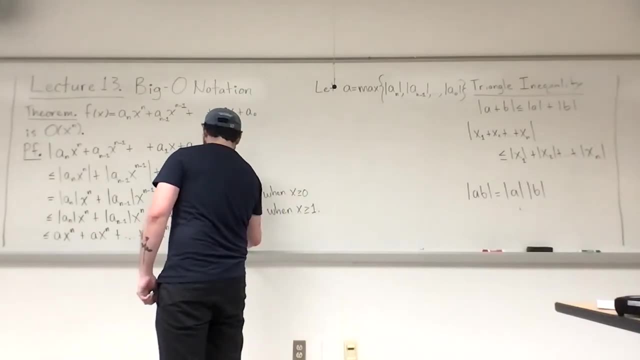 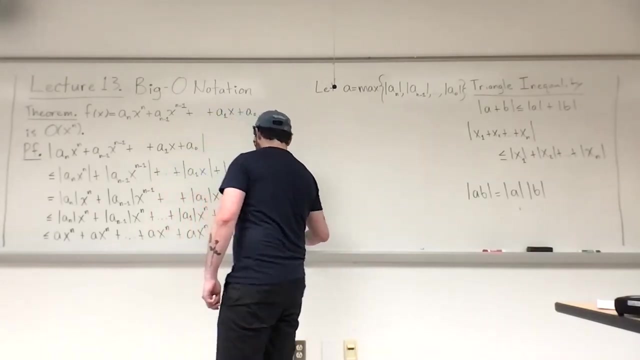 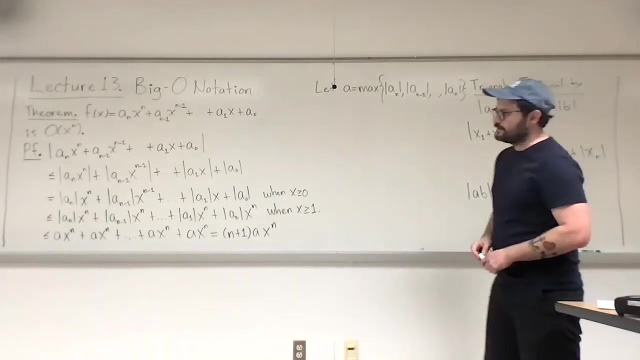 These terms: n plus one of them, Right. So this would be equal to n plus one times A times x to the power n. Again, we're just like see, like making bigger and bigger estimates, but now we have that right. 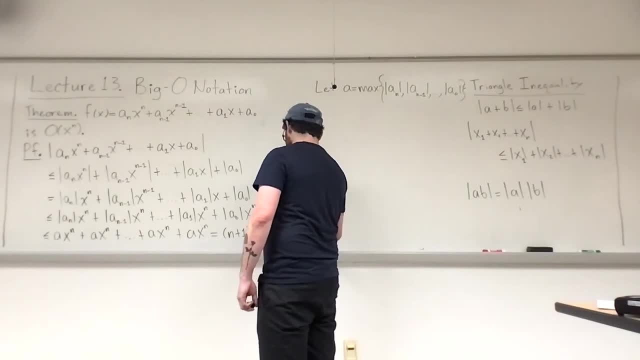 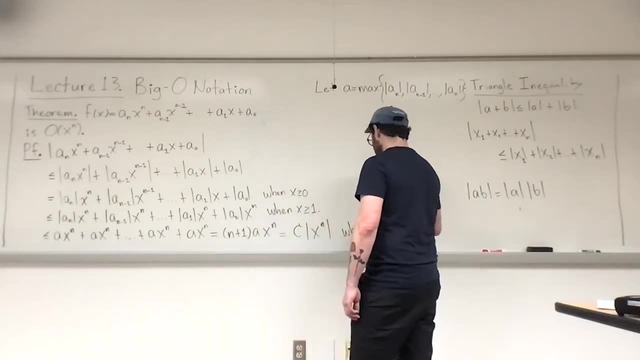 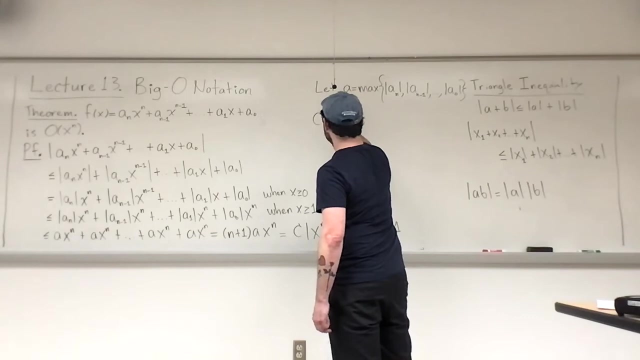 And if you wanted to be clear, And we can write this as: c times x to the value of x, to the power n When x is greater than or equal to one And c is equal to n plus one times a. 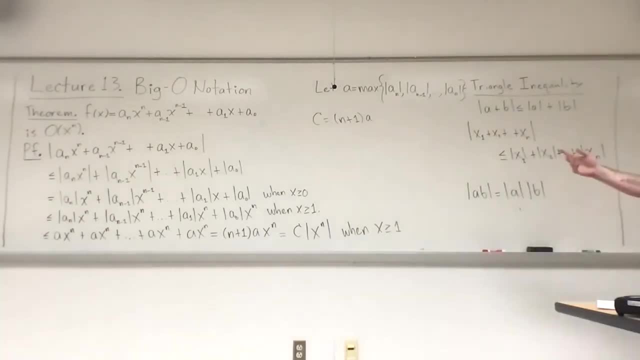 Then there it is. that's a constant. n is a constant, n is a finite number. a is a number, it's a number, so it's a constant. so what did we just show? ran out of order, but like this, is at most constant. 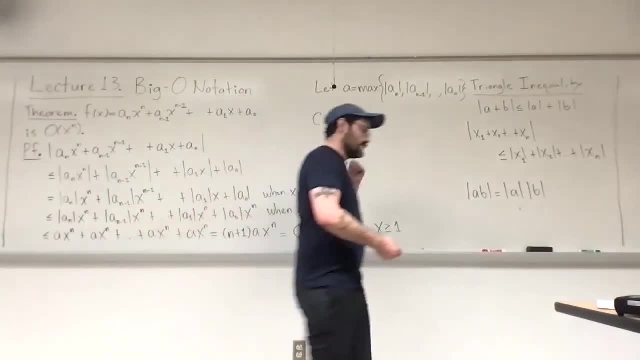 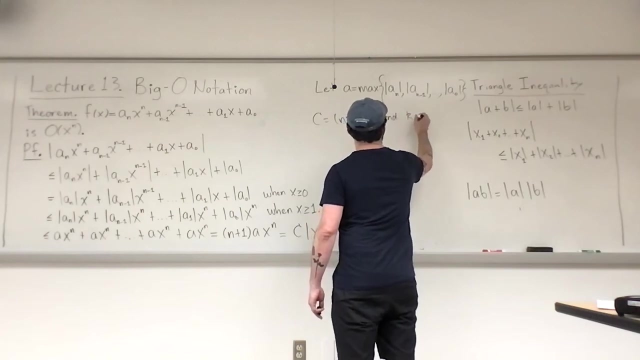 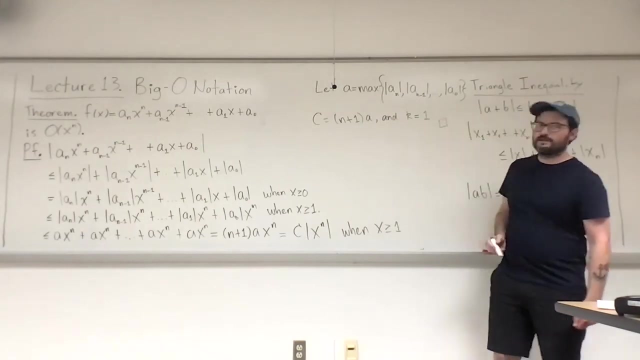 times that, whenever that. Thus That polynomial Is big O of x to the power of n, So it's easy with that. And lowercase k is equal to one. Those are your witnesses, And then It's not like the best looking proof, but that's the idea of. 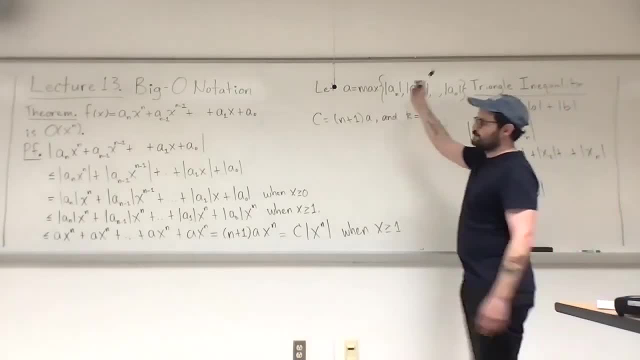 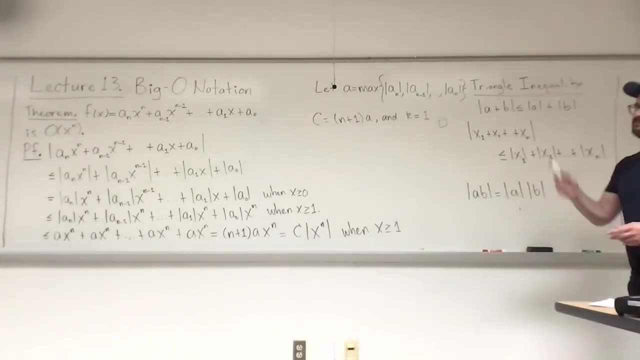 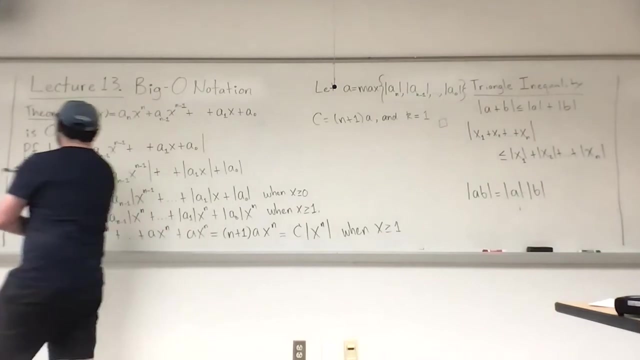 of a vector. Use the triangle inequality, Take the maximum of the absolute values and coefficients, And then by my terms, and then you have a that that only was no more than that and it actually like tells you like what the constant is as well. Any polynomial you have, like you take the max in. 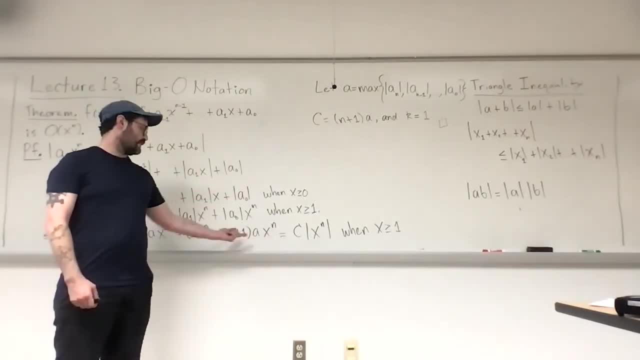 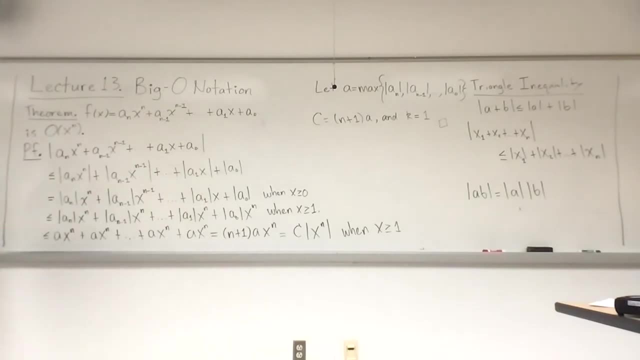 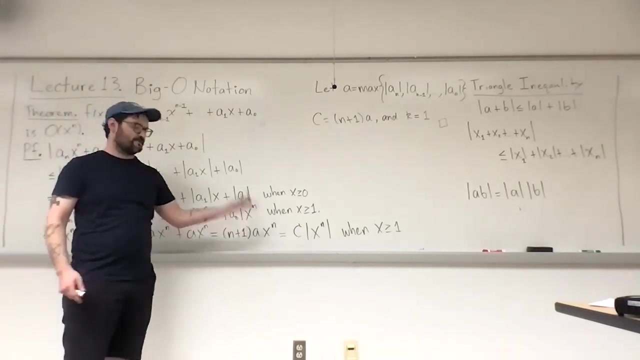 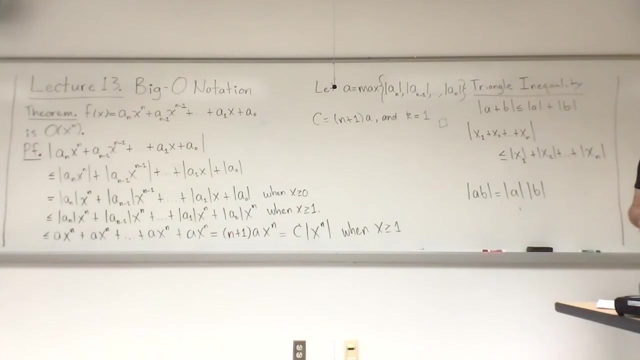 absolute value of all the coefficients and then times that with the degree plus one, that's your c, and then your lowercase k is just one always. So, no matter how complicated that looks, it's no more than just that number times x to the power n. Okay, so now we have a theorem that we can 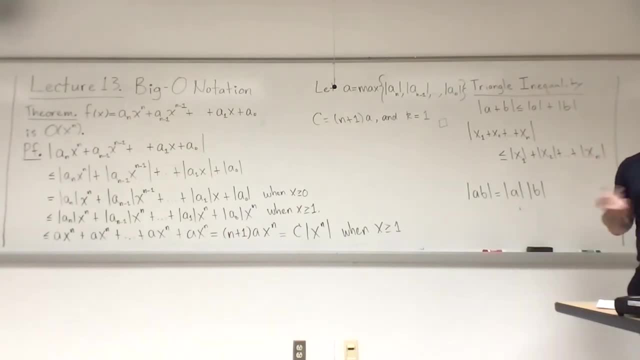 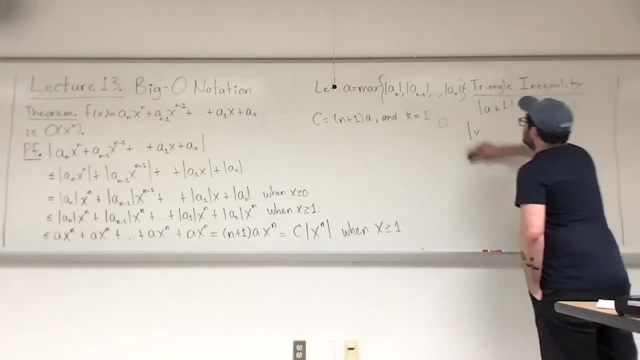 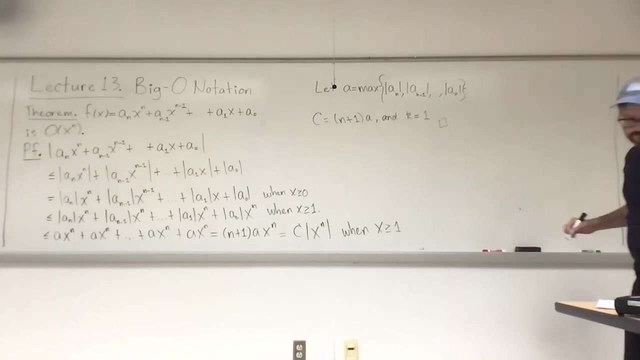 use. whenever we encounter a polynomial, We know immediately the big O estimate for it. Okay, more examples. Let me get a new black marker. That one didn't work. Show. one plus two plus dot, dot, dot plus n is actually instead of show. let's do this without like a target to do. 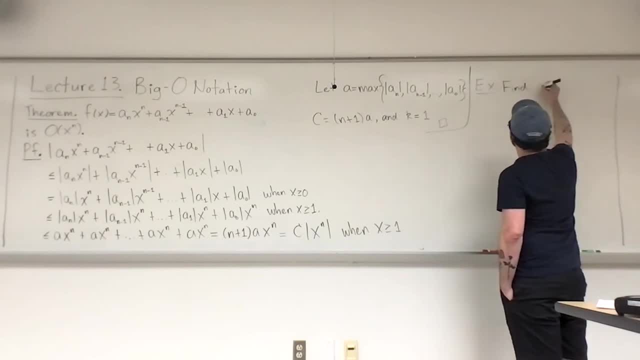 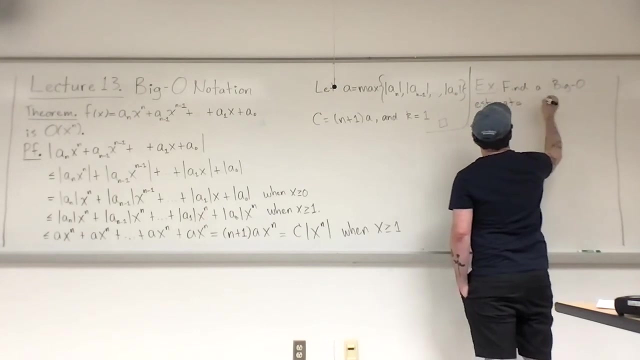 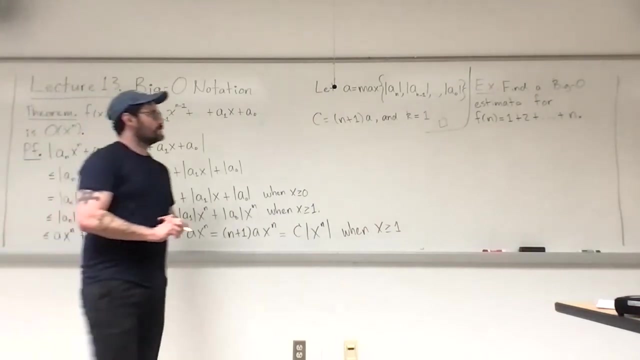 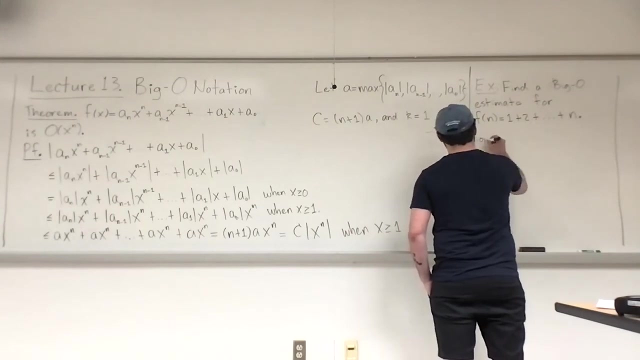 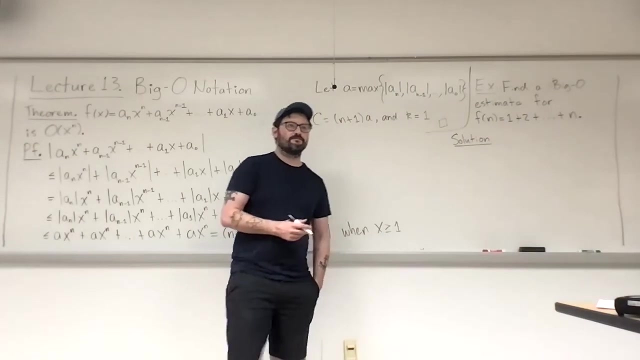 So find a big O estimate, for f of n equals one plus two plus dot dot, dot plus n. So find a big O estimate now, not just like show it to find it Okay. so for this it's actually not so bad. Oh, and whenever you see n, it's typically going to be an integer value function or natural number value. 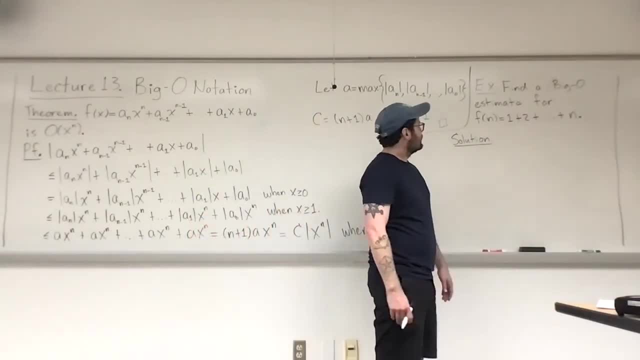 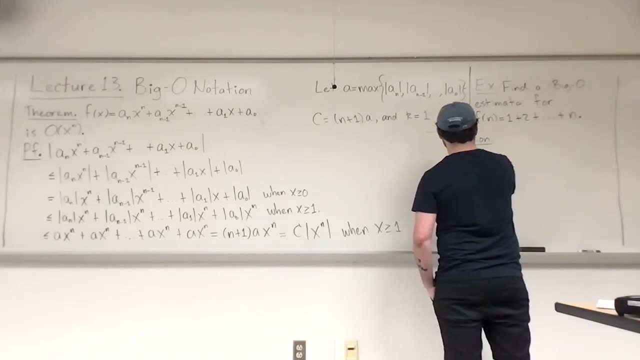 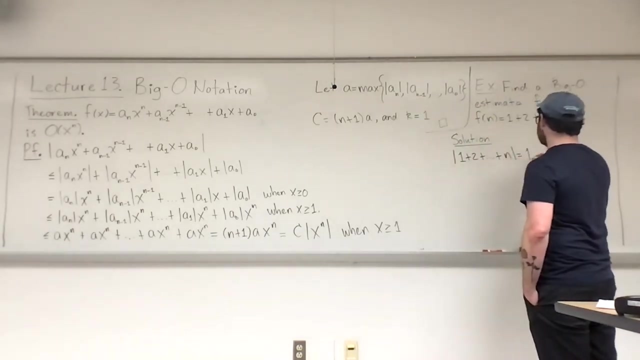 function or input function to me. So n is clearly just positive in an integer. So if you look at the absolute value one four n as n plus two dot dot, dot plus n, that's clearly equal to one plus two plus dot, dot, dot plus n. 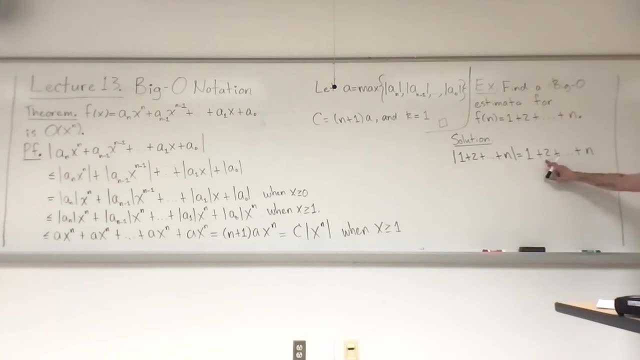 Because it's just positive. It's just positive, Right. But then one less than or equal to two strictly less than two, Right. And two strictly less than x One. they're all strictly less than n, Right. So then I can write: 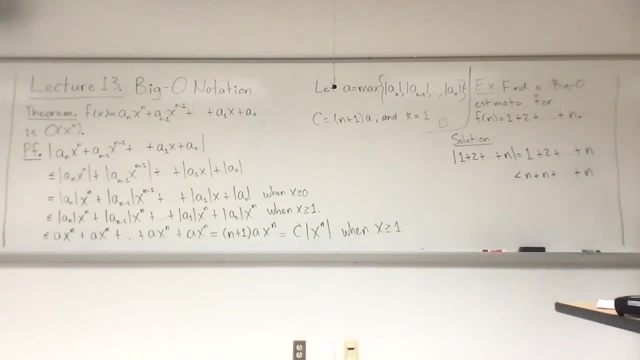 dot, dot plus n. How many n? do we have n of them, right? So this is equal to n times n, right? Oh, wait a minute, Is it the case? I saw one of you wince. How many of them are there? 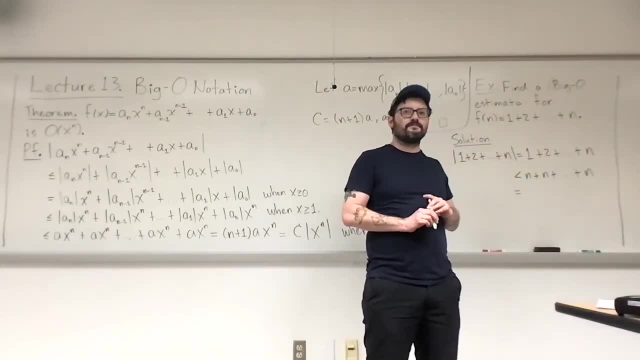 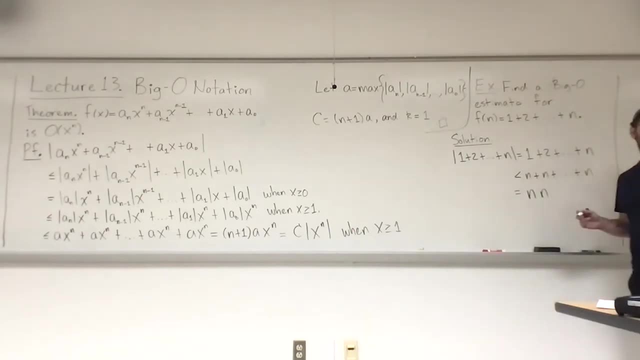 They're just like terms. There's n of them. Yeah, there's n n's, So it is n n's right, Like if there was three n's it would be three times n? right. But we know there's n of them. 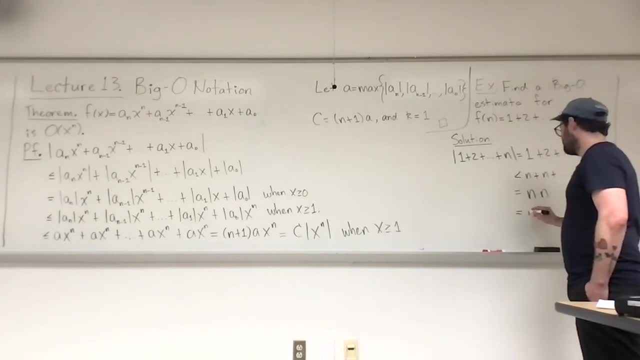 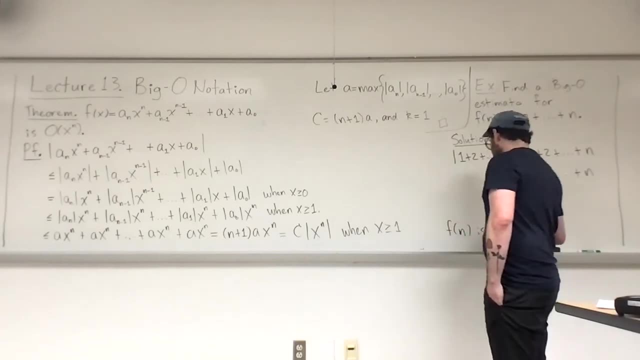 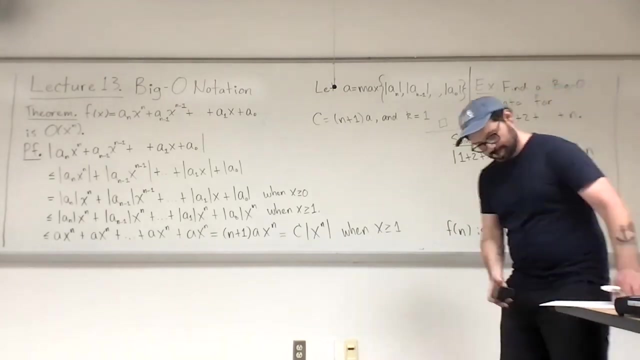 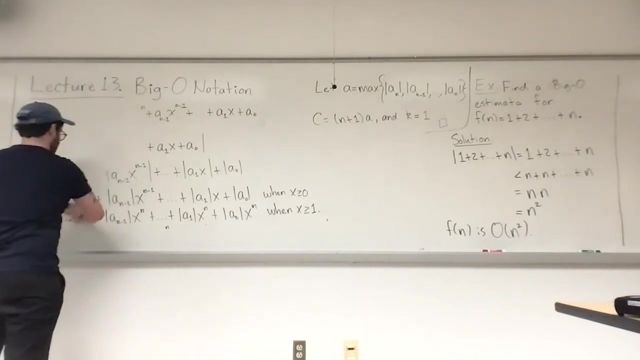 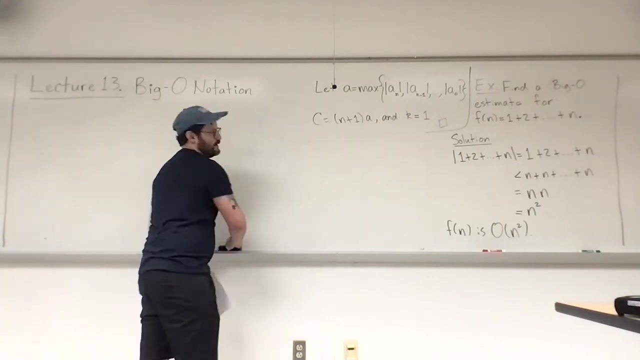 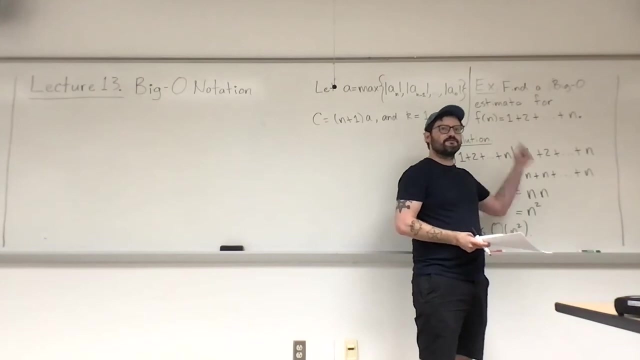 There's n times n. So then this function, here the f of n is big O, but then squared, That's it. And like that type of thing, like, could definitely occur in an algorithm, right, Where, like, for each loop, you do like, you increment one operation, right. 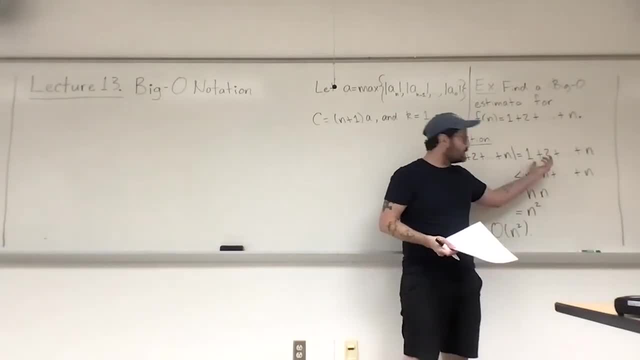 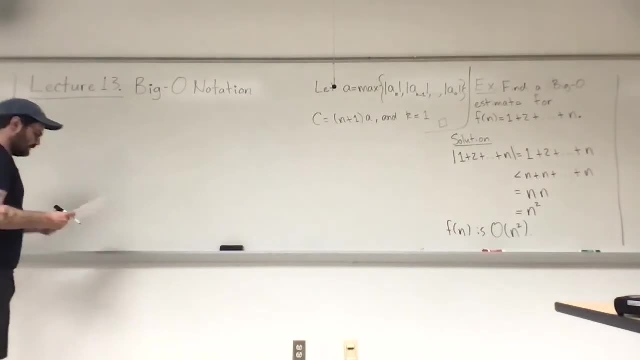 And it's like n loops and you're incrementing n at a time. So this could like measure the number of operations in the algorithm And we'll define that formally next time. Okay, Let's look at another example. So n factorial is: 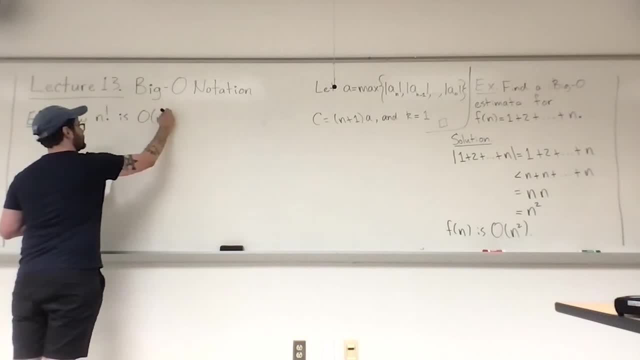 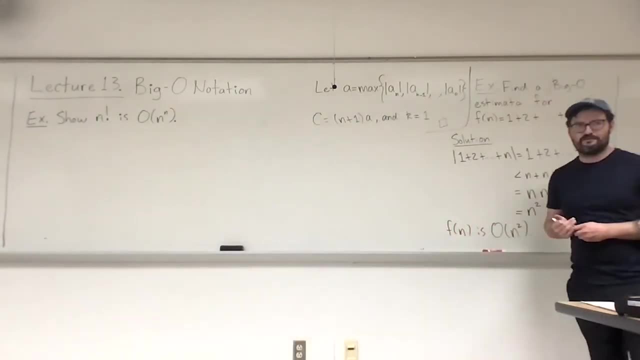 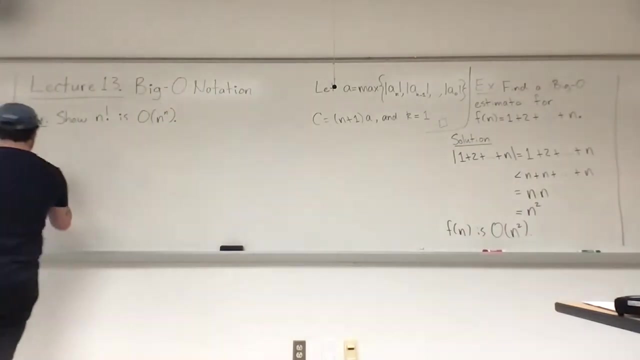 is big O of n to the power n. Have you ever have an algorithm that the number of simple operations is any type of factorial? It's probably a horrible algorithm. Exclusion Factorial is n times n minus one, Times n minus two, all the way down to one right. 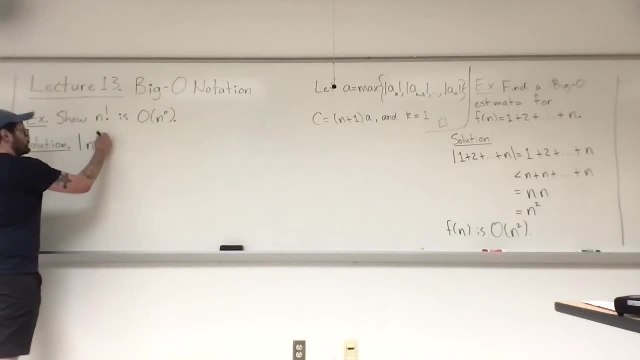 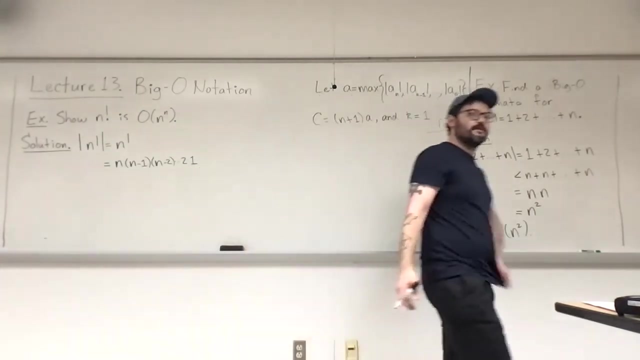 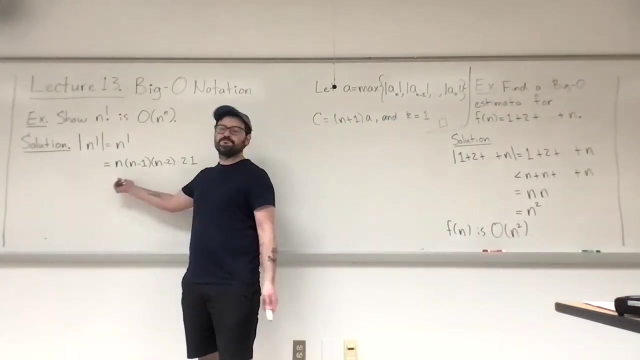 So it's always positive, by the way. So you drop the absolute values. Yeah, that's just the definition of the factorial. Now notice that what's the largest factor here? 10, right, So that's greater than equal to that. 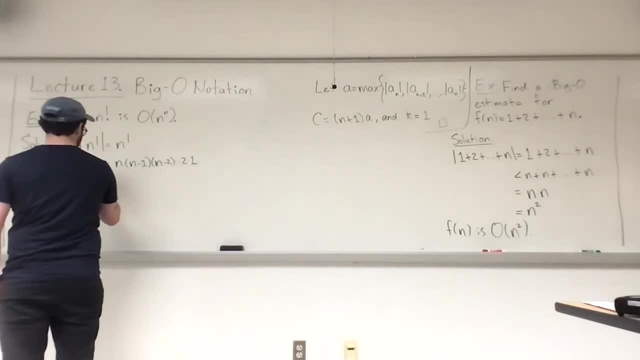 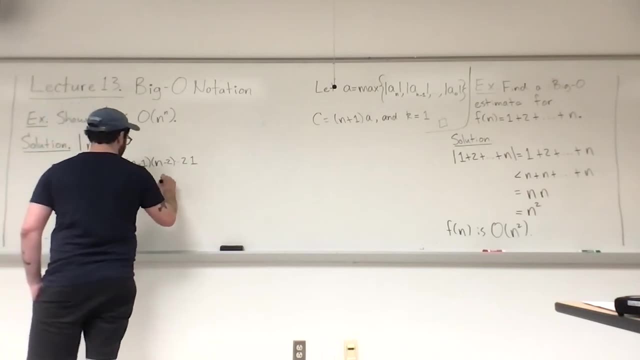 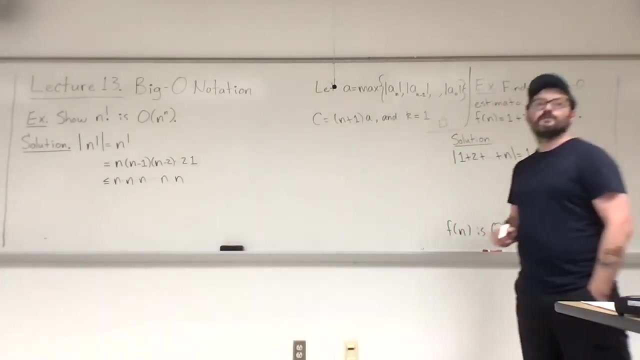 It's also greater than equal to everything following you, right. So this is at most, n times n times n times, dot, dot, dot, times n times n Right, this is it. So you multiply it n, right, in n times. so it's going to be n to the power of n. 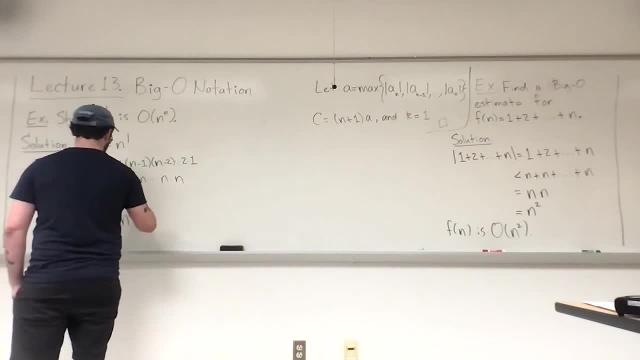 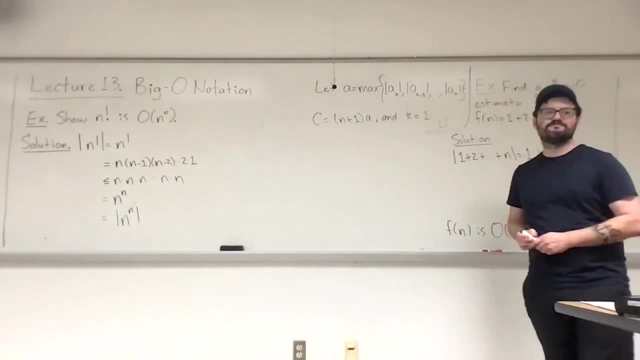 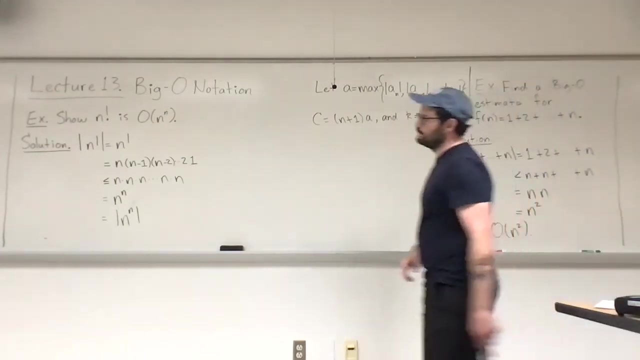 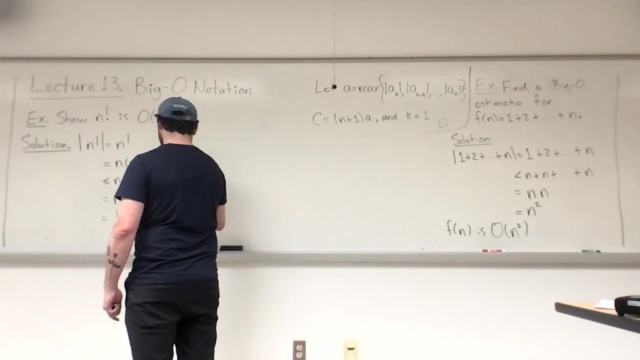 That's obviously equal to the absolute value of n to the power of n. What is t? or is it 2? 2.. Okay, So in particular, what we've just established, really like in general, it's like that's the solution right there, but like we've also established here that in fact, like yeah, n factorial is at most n to the power of n right. 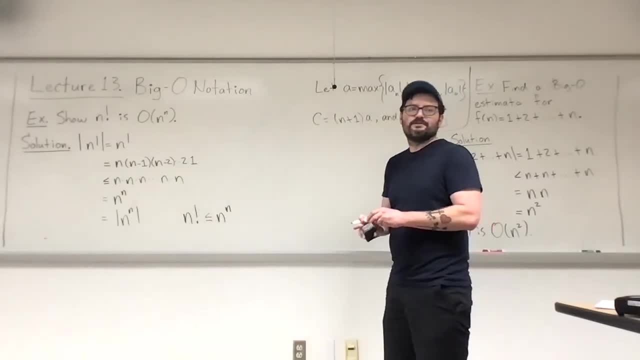 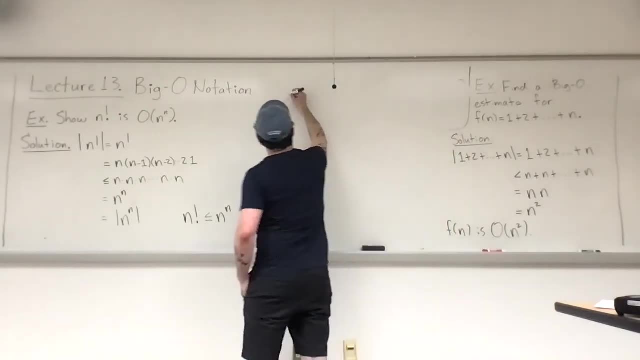 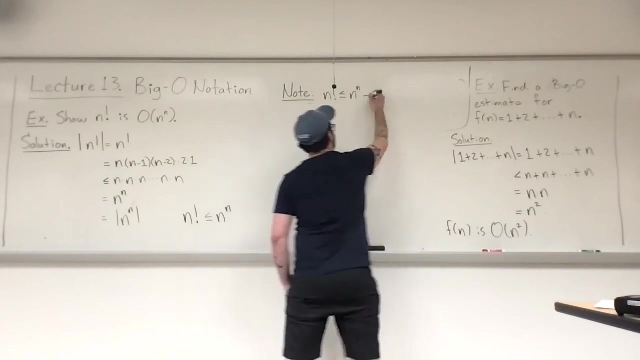 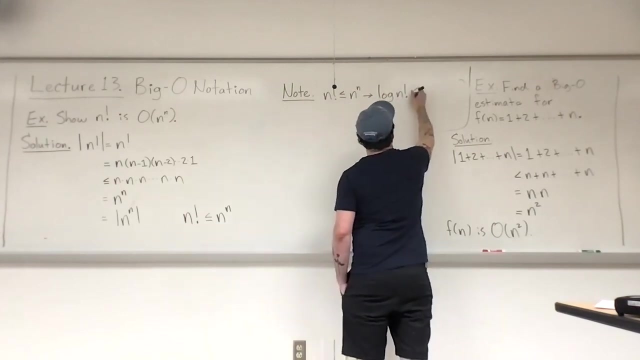 That's what we just established for, like all n right, There's no conditions on there, it's just that right. So I made a note. N factorial is at most n to the power of n implies that log of n factorial is at most log n to the power of n. 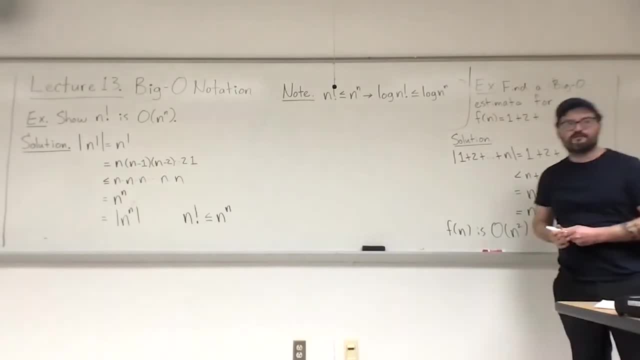 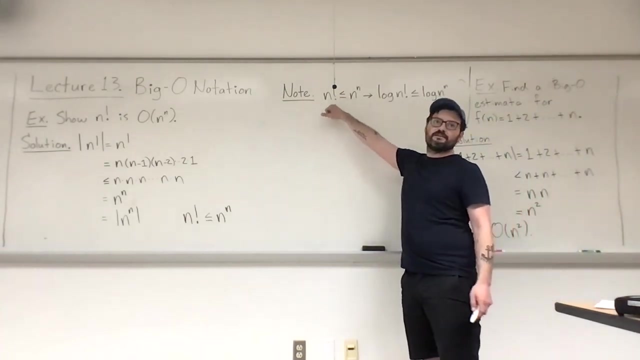 Why is that true? It's only, you can only apply functions on both sides of an inequality when certain things happen. The logarithmic function is increasing right, So it's increasing. so if we apply on both sides right and that's less than that, then log of that is less than or equal to log of that, so it's increasing. 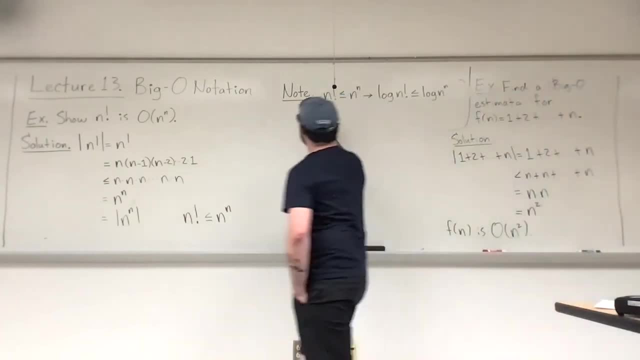 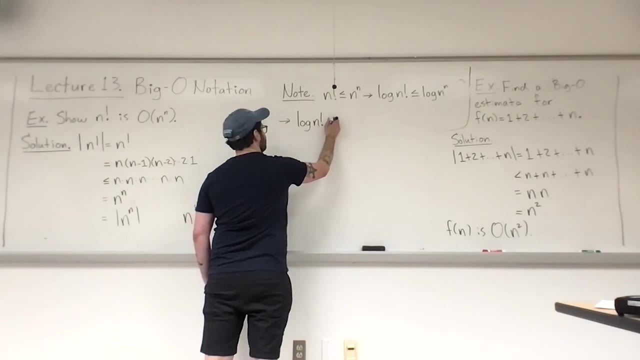 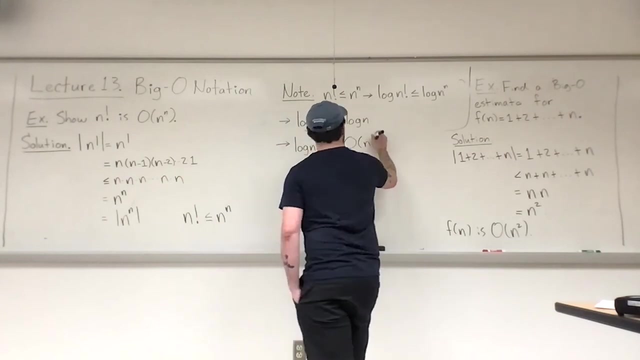 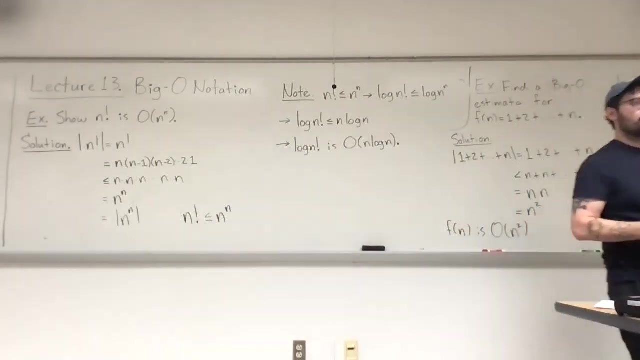 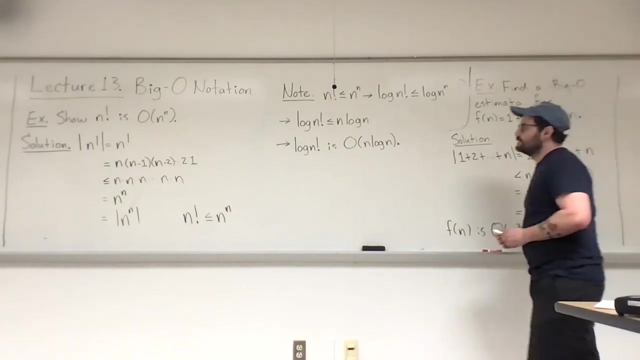 Which this implies that log of n factorial is at most n times log n, Which implies that log n factorial is big O of n log n. So we have like another, we've established another result. So this is a big O estimate on log n factorial. 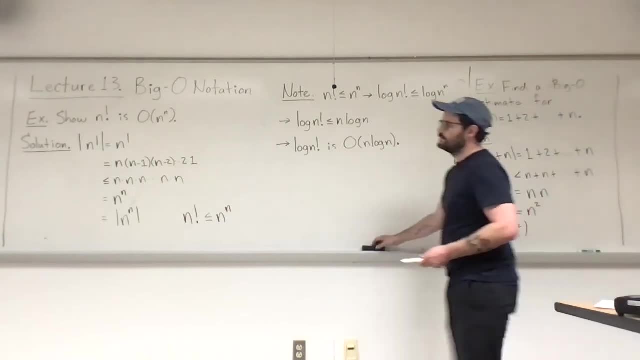 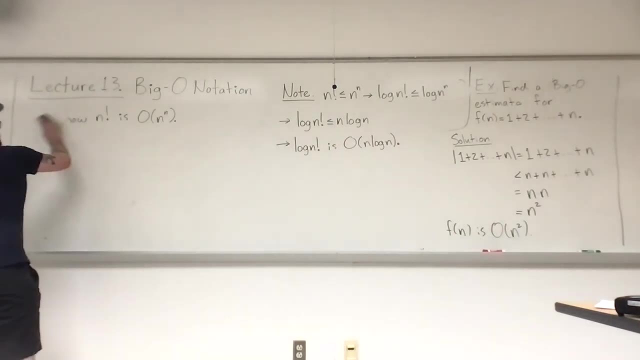 And in many instances, when you're measuring growth of algorithms, you're measuring those, those atomic operations. there is logarithmic growth. It's not like super fast, it's like kind of bendy right. So 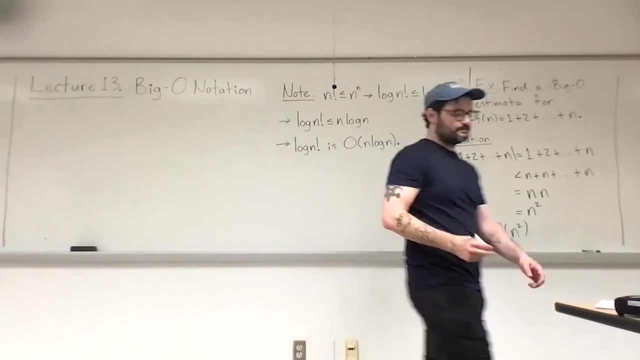 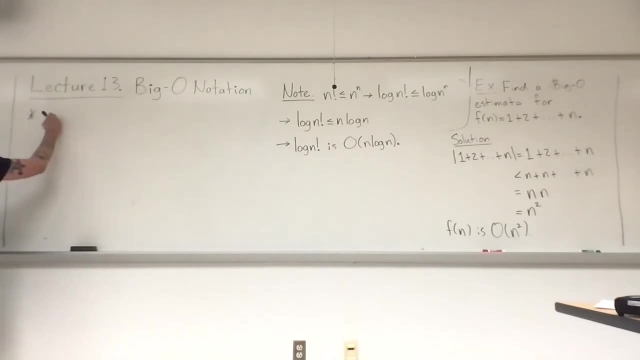 that's why it's important to have, like log estimates on things. And speaking of um, I'll just state a fact that, um, what do I want to say? I want to say, oh, say, I think that's true. 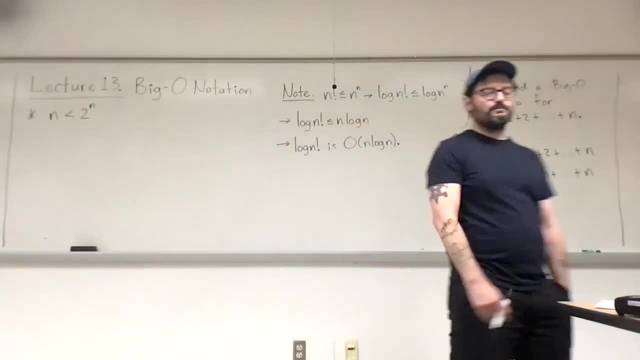 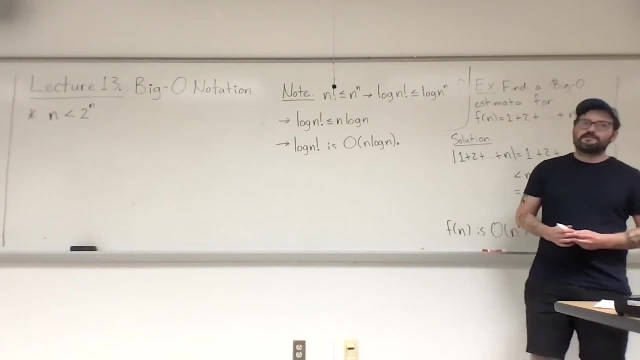 I'm just telling you that that's true. We'll prove it later in the semester, but that's true. We'll prove it later in the semester, but that's true. We're all positive in it, And if you wanted to like verify it with like calculus or something, you could also do that. 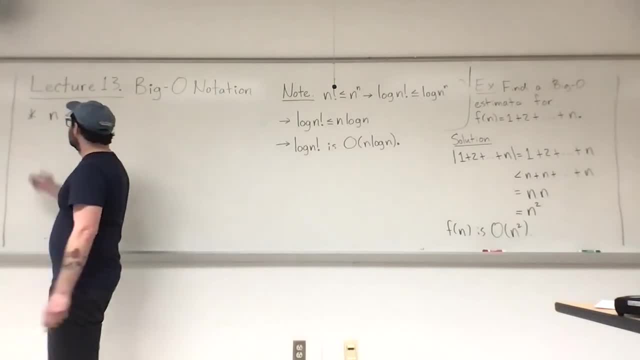 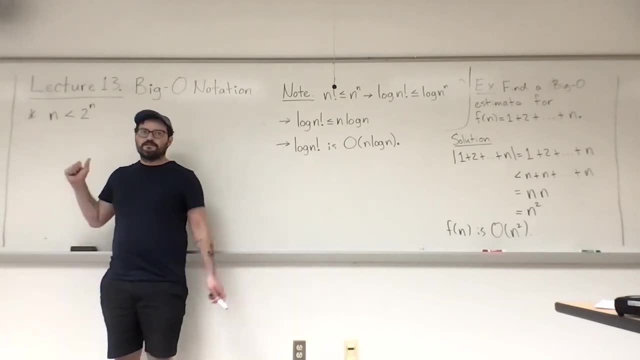 We're going to prove it with something called induction later, But with calculus you can already see it as well. Like just take N to be x and x is positive, right. And then just evaluate like okay, put x to be like 1, right. 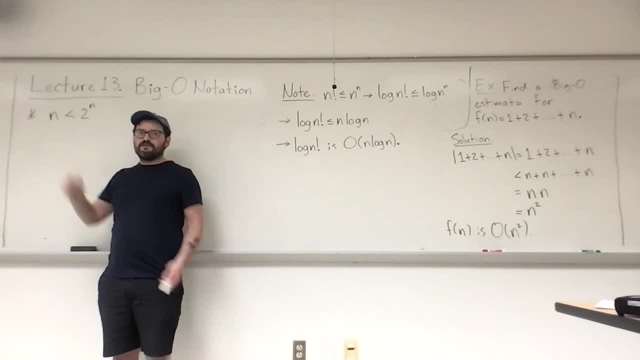 So then 1 is less than or equal to 2.. Good, And then look at the rate of change. Take the derivative. On the left-hand side you have a constant rate of change change, and on the right hand side you have a growing rate of change, so that one's always.